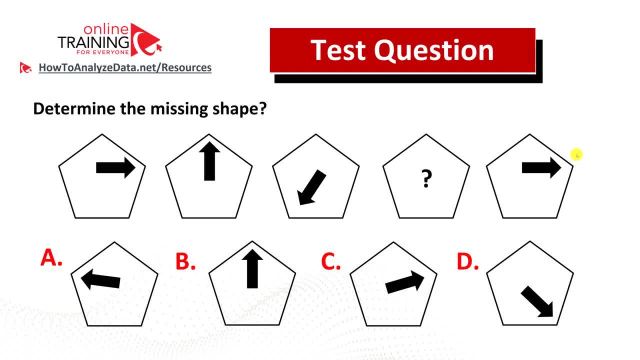 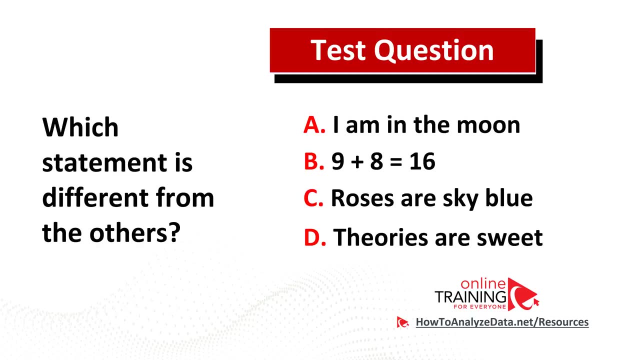 represented in the original question. Hopefully, you've nailed this question and maybe even figured it out, And I hope that my instructions give you ability to answer these types of questions in the test. And now here's the question for you to try. Please make sure to post your answers in the comments. 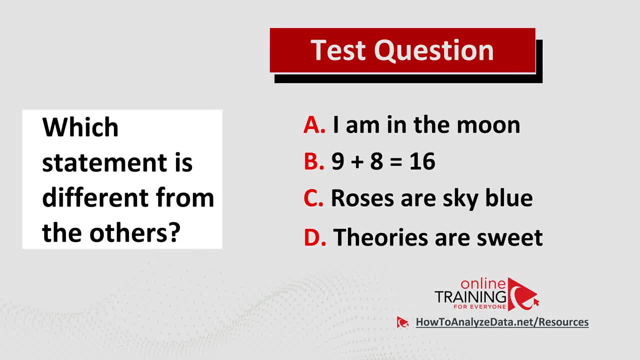 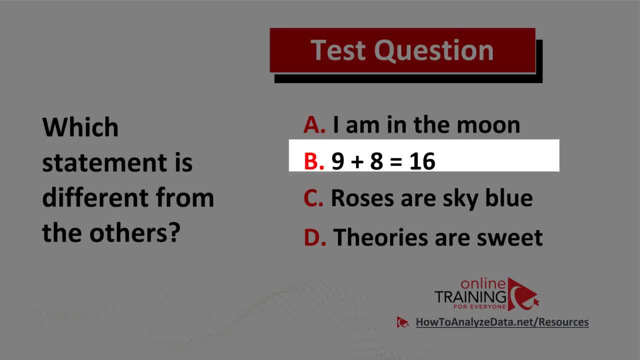 section of this video so I can give you my feedback. Which statement is different from the others? The first statement: A- I'm in the moon. Choice B: nine plus eight equals 16.. Choice C: roses are sky blue And D- theories are sweet. Do you think you know the answer? Feel free to. 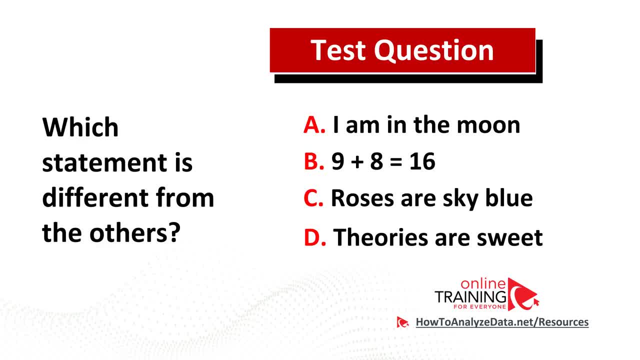 pause this video and try to solve it, And if you came up with the answer, feel free to post it in the comments section of this video so I can give you my feedback. Thanks for participating. One comment is: roses can be blue. Please search on Google blue roses and you will see the picture. 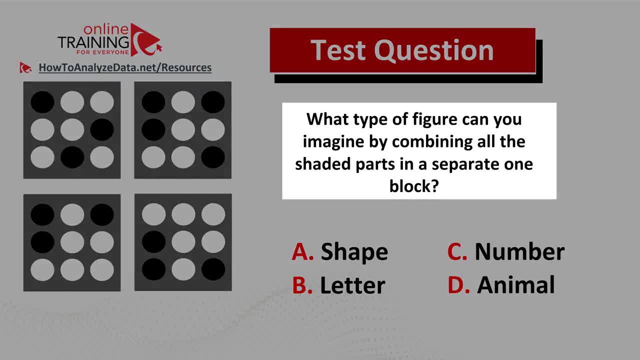 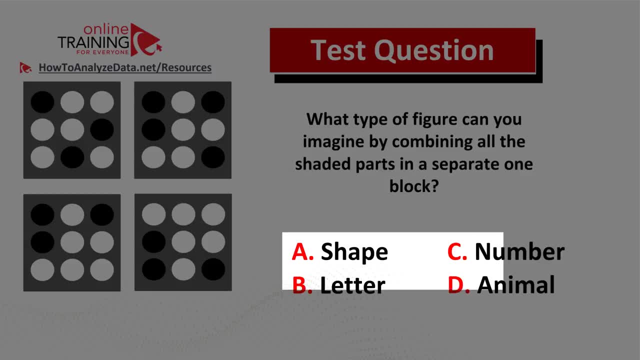 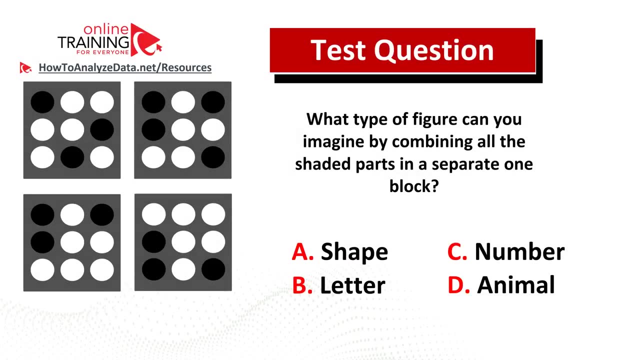 Here's the tricky question from the real test: What type of figure can you imagine by combining all the shaded parts in a separate one block? And you have four different choices: shape, letter, number or animal? Do you think you know the answer? Now might be a good time to answer. 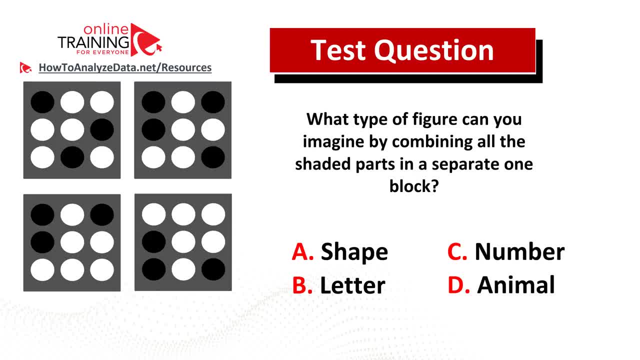 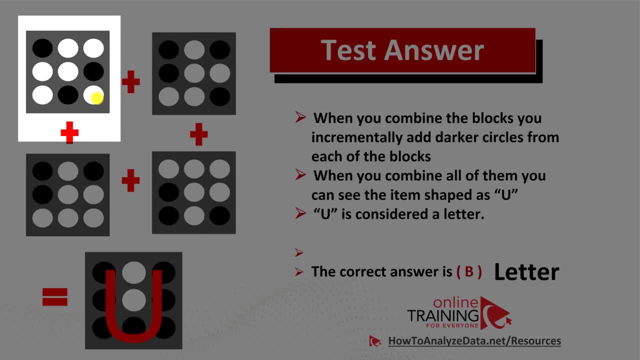 Have a good one to pause this video to see if you can come up with the answer on your own. Did you come up with the answer? Let's see how we can solve this challenge and get to the solution together. The tricky part here is combining all four blocks right in your memory and using your imagination to come up with 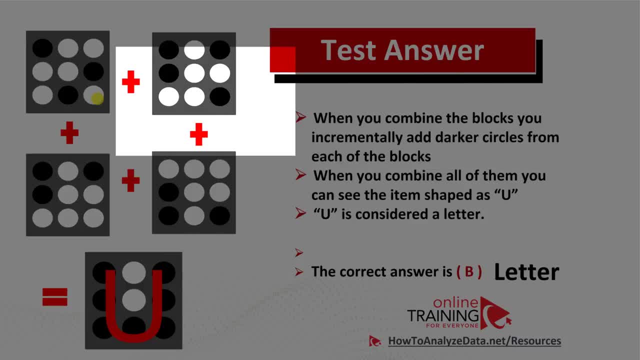 the final answer. But when you combine the blocks incrementally, you add darker circles into one single image And final image here in the sequence represents all darker circles added in one image And, as you can see, the shape of the darker circles represent letter U, So the 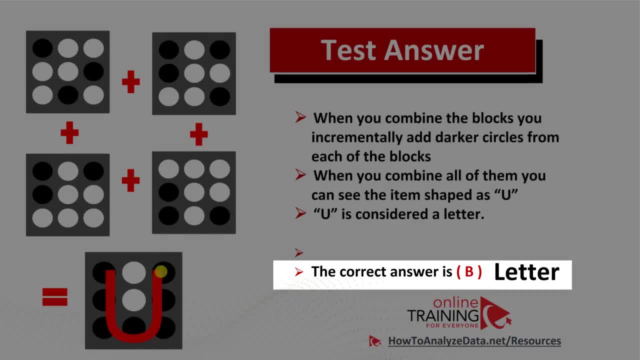 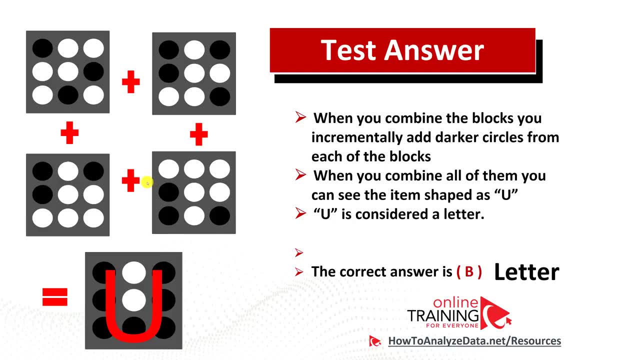 correct answer. here is choice B letter. Hopefully you've nailed this question and now know how to answer these types of questions in the test. But in case you need more questions or practice problems, please make sure to check out my aptitude test ebook in the description section of this video. 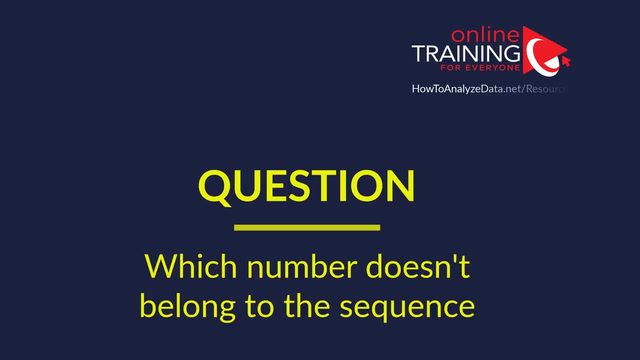 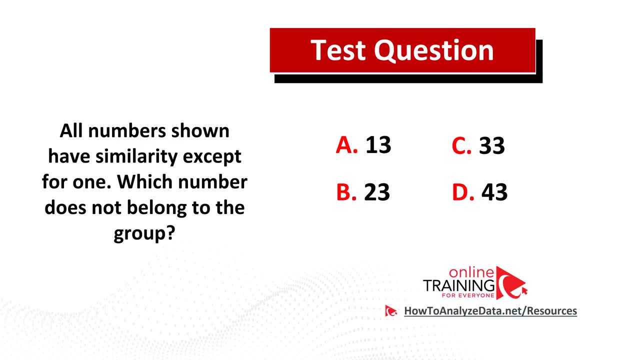 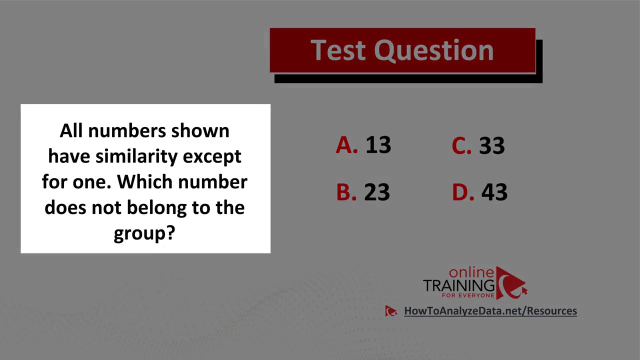 Some of you might find this question tricky, but regardless of whether you can solve it or not on your own, you will be excited to learn the solution to this real-life assessment test question. All numbers shown have similarity except for one, Which number does not belong to the group And? you have four different choices: Choice A: 13., Choice B: 23.. Choice C: 33. And choice D: 43.. Do you think you know the answer? If you do, please let me know in the comments, And if you don't, please. 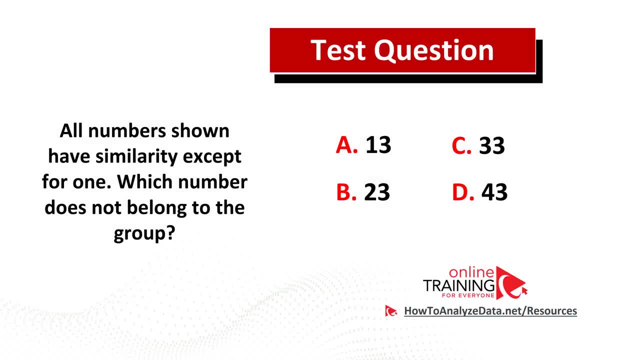 let me know in the comments below. Now might be a good time to pause this video to see if you can come up with the answer on your own. Did you come up with the answer? Let's continue to see how we can solve this challenge together. The solution lies in understanding very simple math concept. 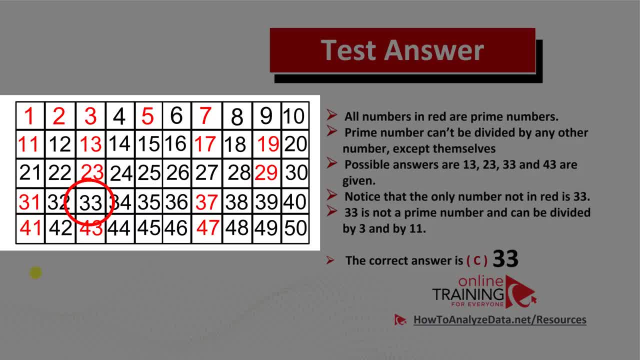 the concept of prime numbers. You see on the left the grid of numbers from 1 to 50.. And all the numbers that are considered prime numbers are highlighted in red. What is prime number? Prime is the number that you can only divide by itself. You cannot divide it by any other number. For. 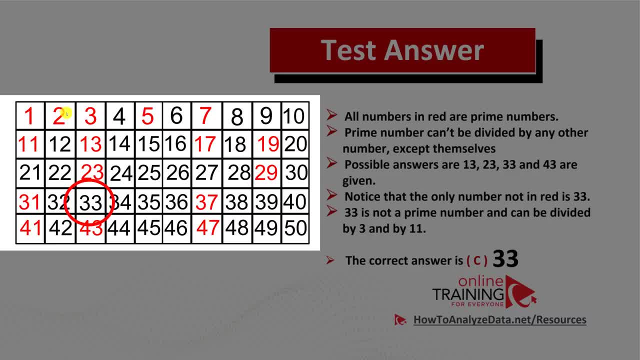 example 1, you cannot divide by anything but 1.. Same for 2,, 3,, 5,, 7, and etc. Out of all the numbers presented in the question, 33 is not a prime number, Because 33 can be divided by 3 and also. 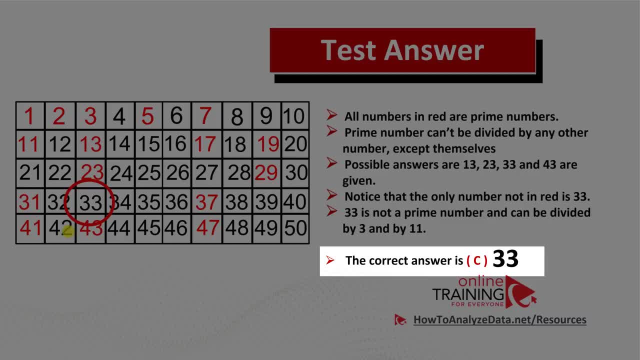 can be divided by 11.. So the correct answer here is choice C 33.. Let's recap: All numbers in red presented in the grid are prime numbers. Prime number cannot be divided by any other number except themselves. Possible answers are 13,, 23,. 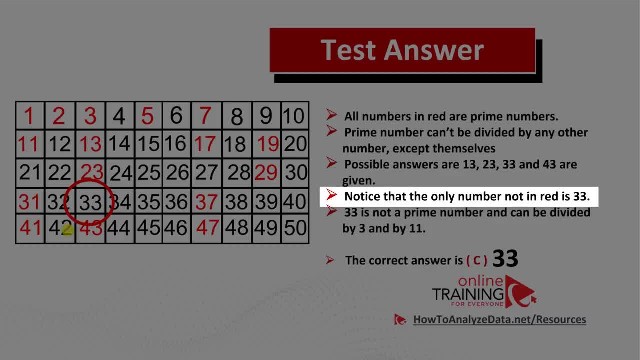 33, and 43. And the only number that is not a prime number is 33.. 33 is not a prime number because it can be easily divided by 3 and by 11. So the correct choice here is choice C 33.. 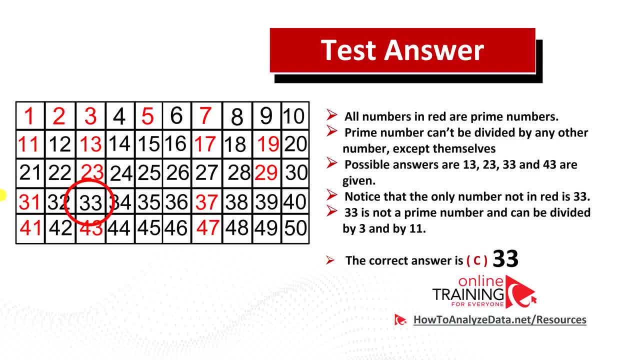 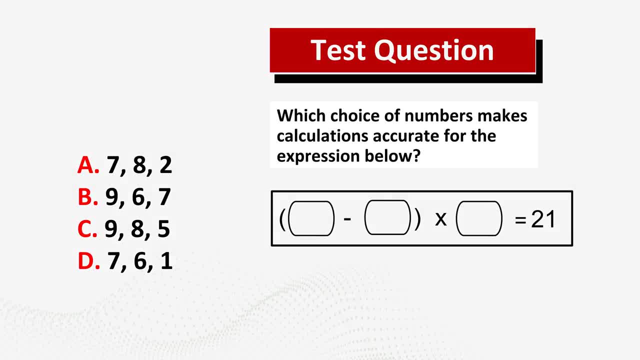 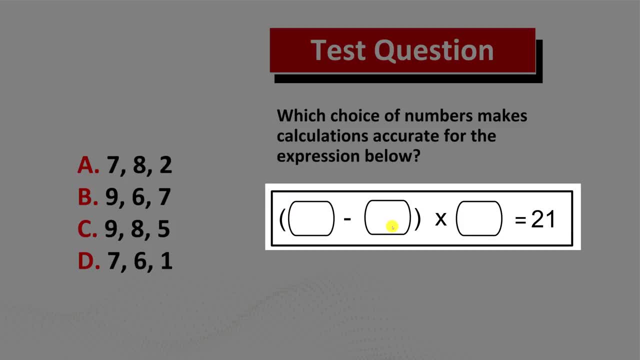 Hopefully you've nailed this question and now know how to answer these types of questions on the test. And now here's the question for you to try: Which choice of numbers makes calculations accurate for the expression below? And you have an expression: Two numbers in parentheses multiplied by a third. 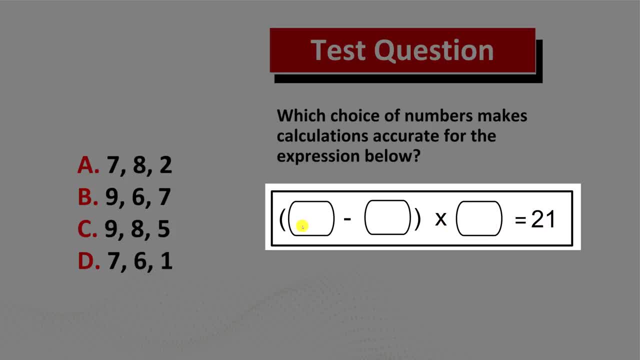 number equals 21.. And for two numbers in parentheses you subtract second number from the first number And you have four different choices: Choice A- 7, 8,, 2.. Choice B- 9, 6,, 7.. Choice C- 9, 8,, 5. Or choice D. 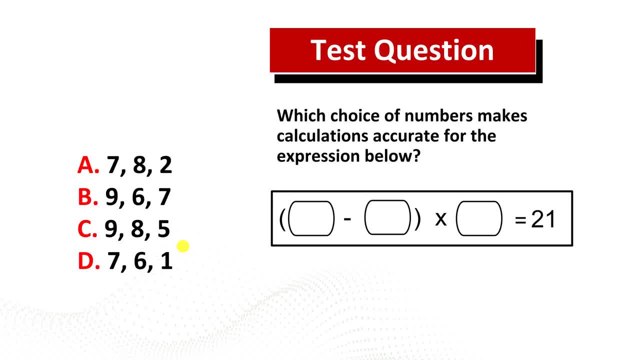 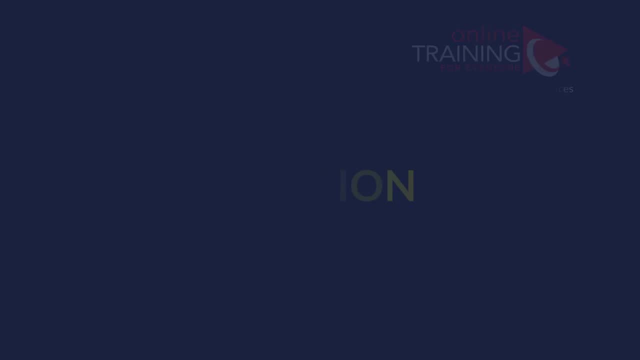 7, 6, 1.. Feel free to pause this video and try to solve it And if you came up with the answer, feel free to post it in the comment section of this video and I'll give you my feedback. Thanks for participating. Here's the tricky question from the real test, But somehow I 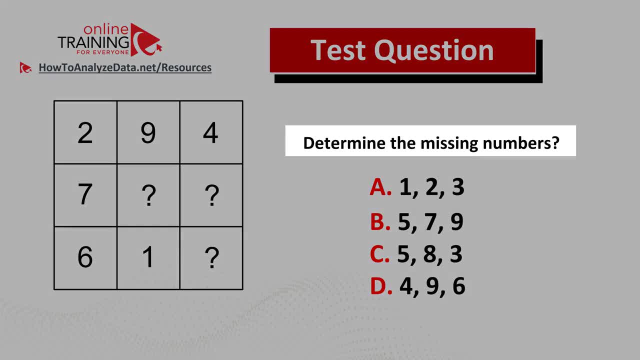 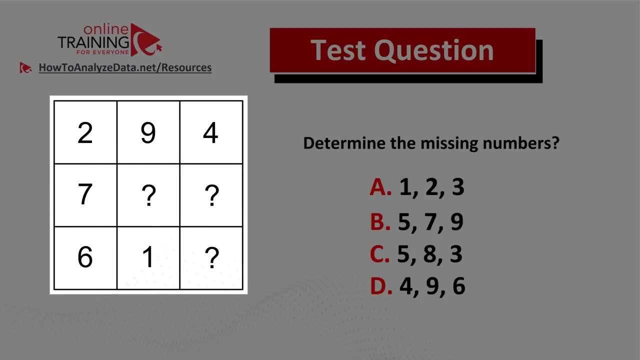 have a feeling that you might come up with the answer: Determine the missing numbers, And you have a square which has nine numbers And three out of nine numbers are missing And you have four different choices: Choice A: 1, 2, 3.. Choice B: 5, 7, 9.. Choice C: 5, 8,, 3.. And 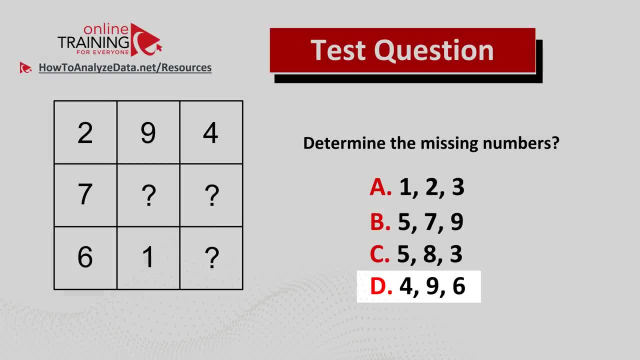 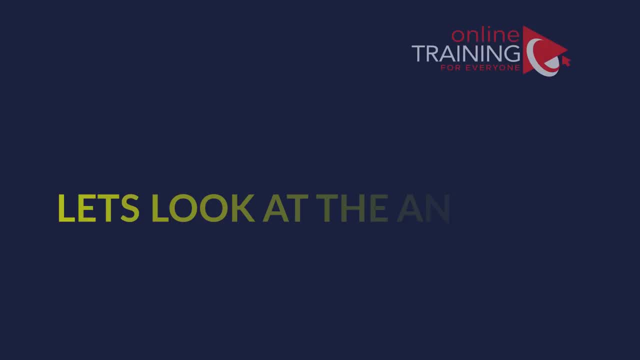 choice D, 4,, 9, and 6.. Do you think you know the answer? Now might be the right time to pause this video to see if you can come up with the answer on your own. Did you come up with the answer? Let's. 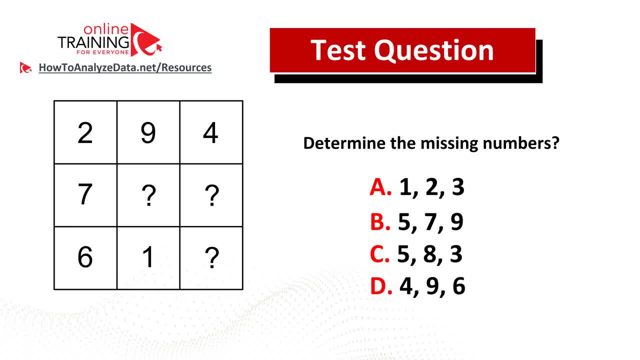 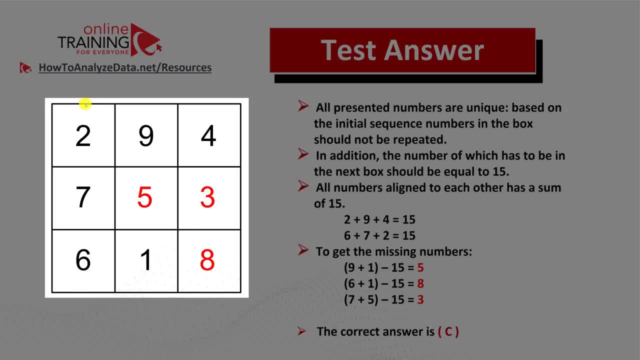 continue to see if we can solve this challenge and get to the correct solution together. There are a couple of things going on. How is this square? First of all, all presented numbers are unique. You can just determine the missing numbers by finding the numbers that are not presented yet on the square. Second pattern: 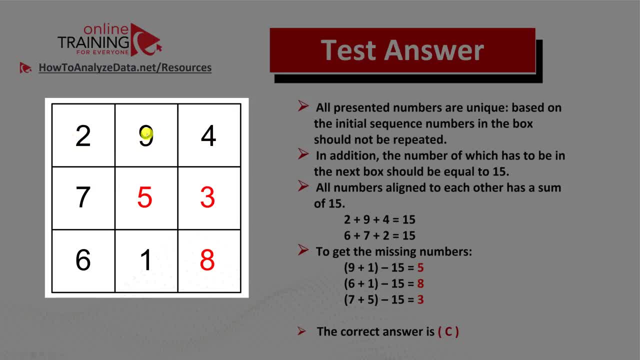 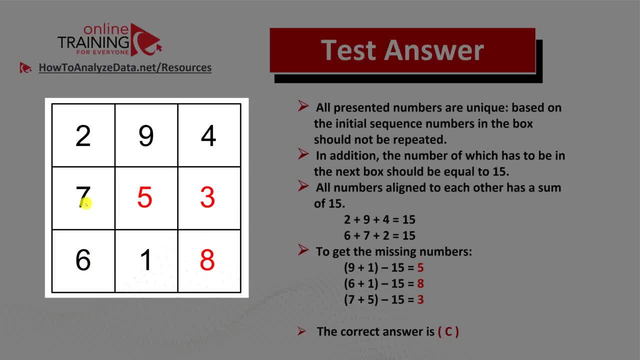 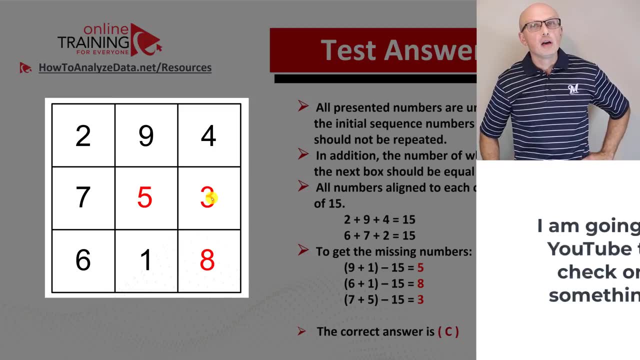 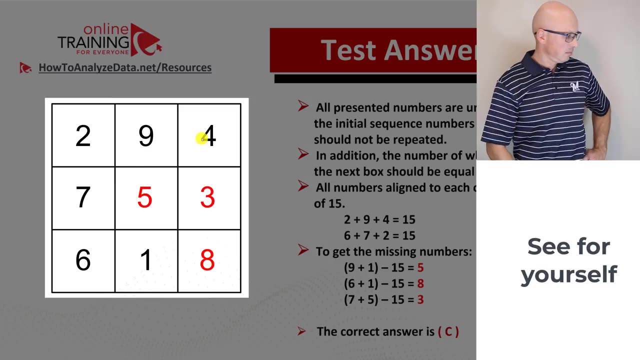 So you can pick the numbers based on this knowledge and find the missing numbers based on uniqueness, and put them in the right places based on the second pattern that we see. Funny thing is you also see that diagonally numbers also add up to 15.. 2 plus 5 plus 8 is 15.. And then 4 plus 5 plus. 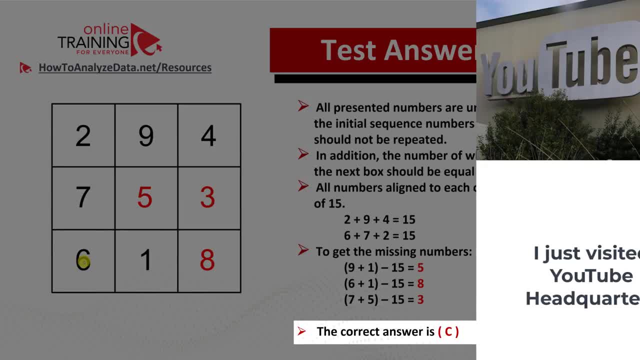 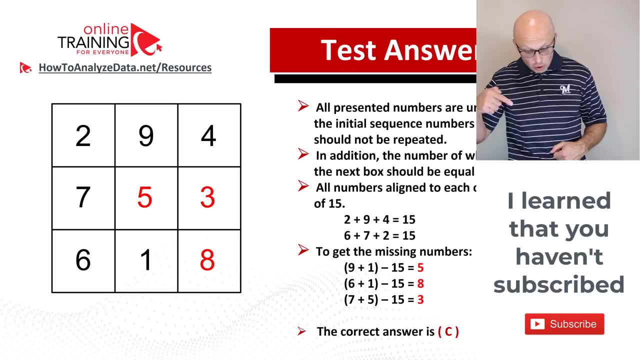 6 is also 15.. So the correct answer here is choice C, And the missing numbers are 5,, 3, and 8.. Hopefully you've nailed this question on your own, Or if you didn't learned how to answer similar questions in the test, But in case you need more, 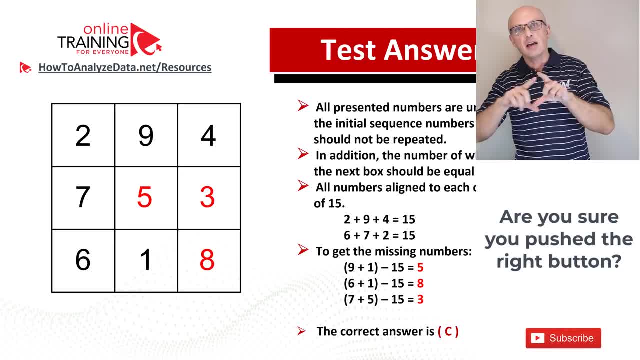 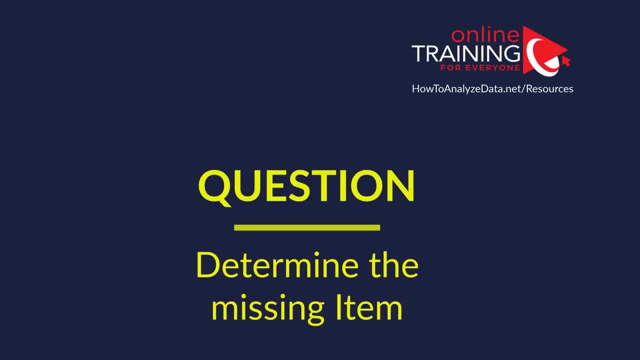 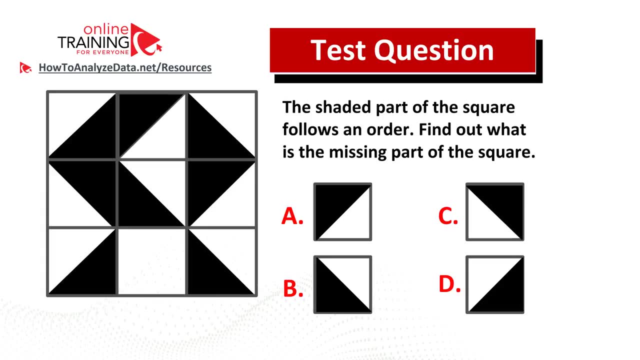 questions or practice problems. please make sure to check out my ebook in the description section of this video. The question here is quite tricky, but I would like to show you the solution which, as you will see, is quite simple: The shaded part of the shade. follow the order, Find out what is. 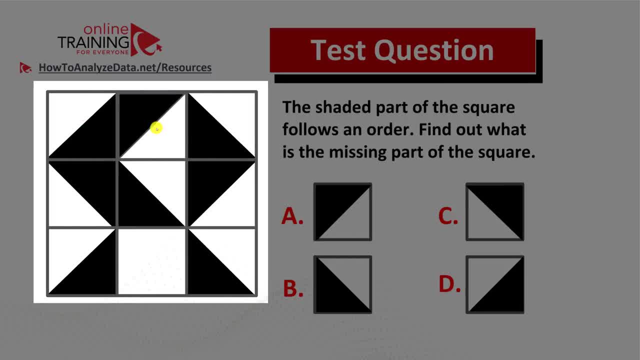 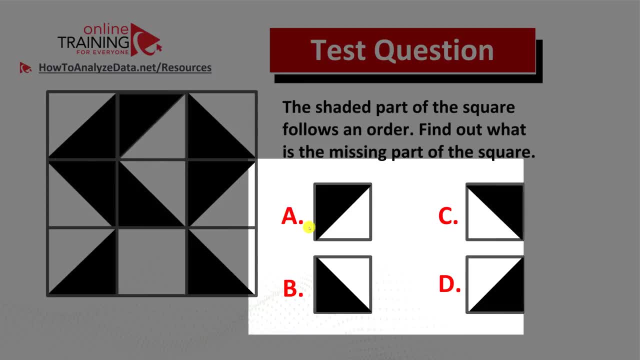 the missing part of the square And you are presented with the 3x3 square And one box inside the square on the lower part in the middle is missing. You need to pick a replacement square out of four possible choices. Choice A: 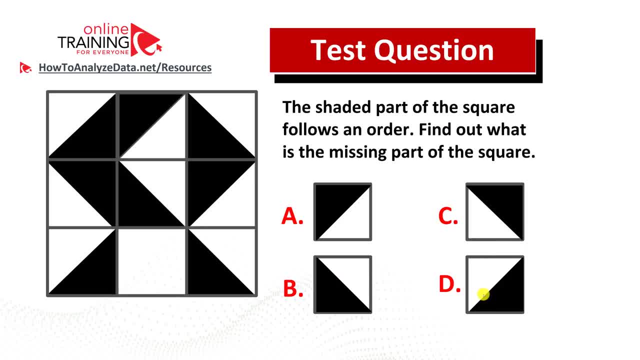 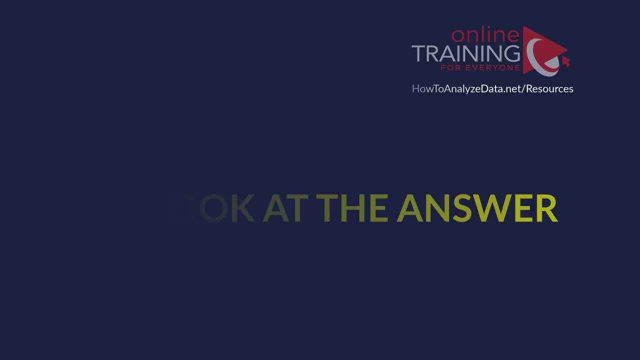 B, C and D. Do you think you know the answer? Now might be a good time to pause the video to see if you can come up with the solution on your own. Do you think you know the answer? Let's continue to see how we can solve this challenge together. 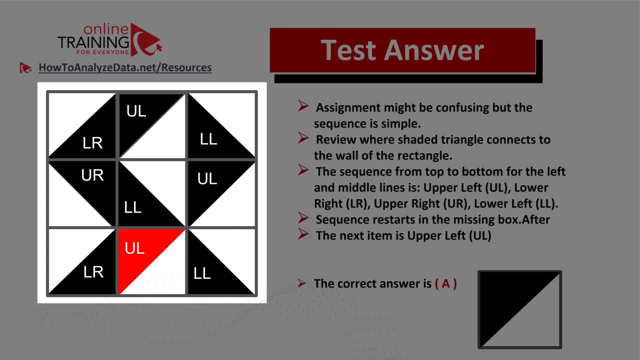 And get to the correct answer. As usual, to solve these types of questions you need to look at the sequence, And sequence is determined by where inside dark triangle connects to the inside walls of the rectangle. So, for example, if you look at the left and middle line, this is where the sequence is. You see that it. 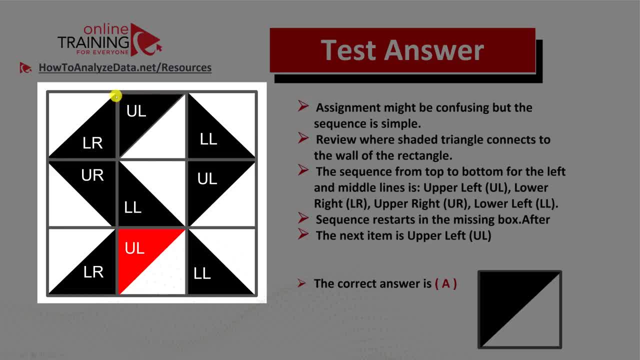 starts with upper left, So we have upper connection and then left connection, Then goes to lower right, So we have lower connection and then right connection, Then goes to upper right connection, And then this is the missing box where we need to find the missing square. And you see that the 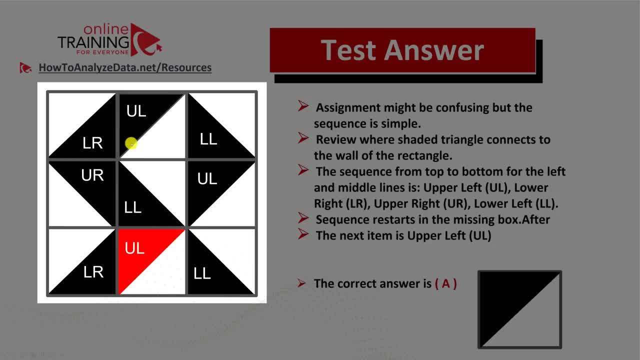 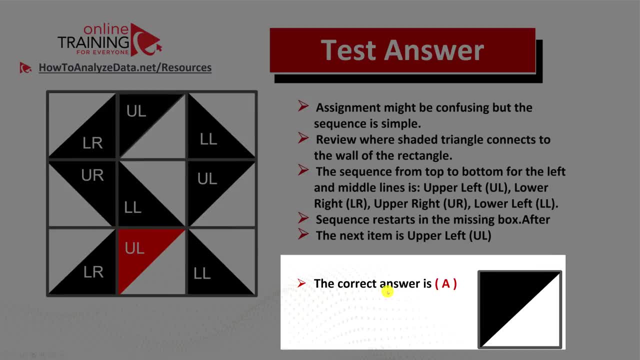 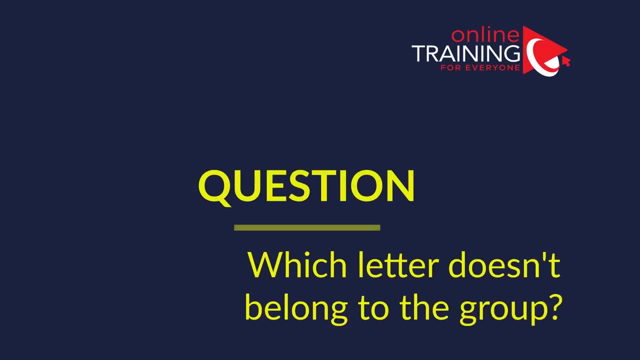 pattern here is starts: Upper left was the first item in the sequence, So the next item in the sequence would be upper left again. So the correct choice here is choice a- upper left. Hopefully you've nailed this question. Do you have questions about showed topics? Some of you might come to the next part of this quiz and tell us which topic you choose. Give and wait till the next part of this next video. Dr Sam з skeпер Subtitles'll let everybody know which topic you make sure you check, without leaving the question box. Jeżeli kimse Brisbane, то אל вам dallaj забол увидеть его на ютубе. Some of you might come to the next part of the video. if you have any questions about showed topics, viene. 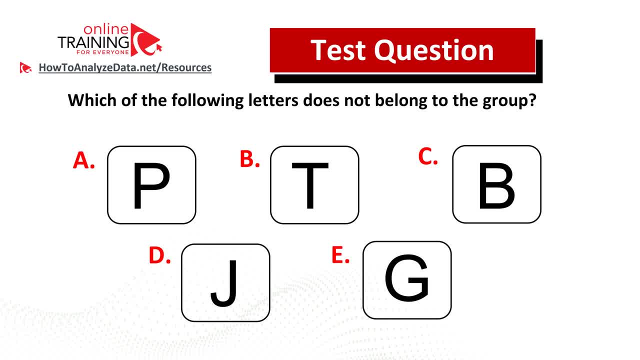 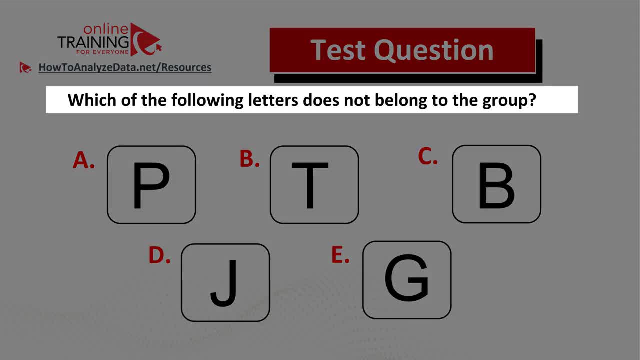 find this question tricky, but regardless of whether you can solve it or not on your own, you will be excited to learn the solution to this real-life assessment test question. Which of the following letters does not belong to the group? And you have five different choices. 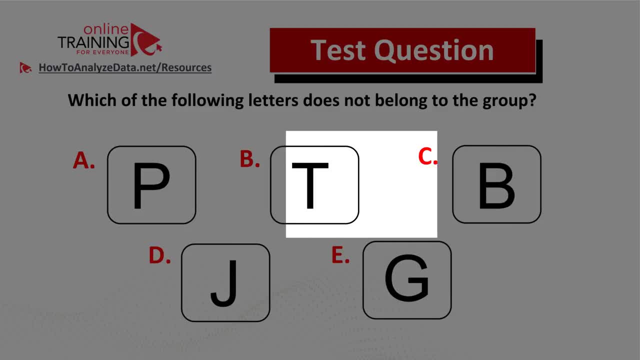 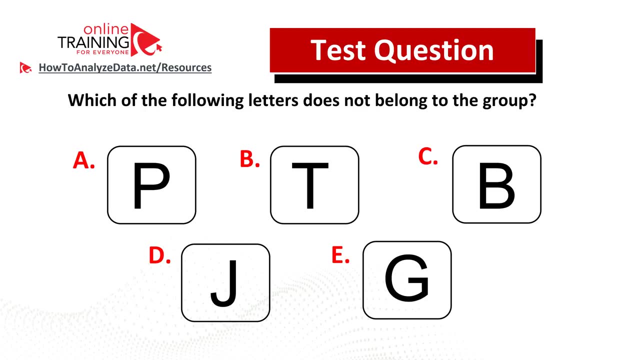 Choice A- letter P, Choice B- letter T, Choice C- letter B, Choice D- letter J And choice E- letter G. Do you think you know the answer? Now might be a good time to pause this video to see if you can come up with the answer on your own. 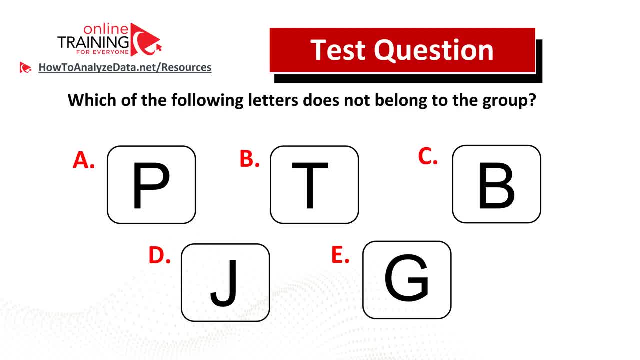 Let's continue to see if we can solve this challenge and get to the solution together. Before we jump to the solution, I would like to give you a clue: Always look for patterns, And the pattern here might be sharp edges versus rounded areas for the letters. 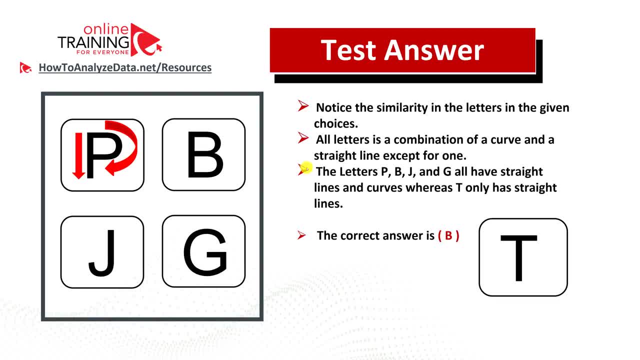 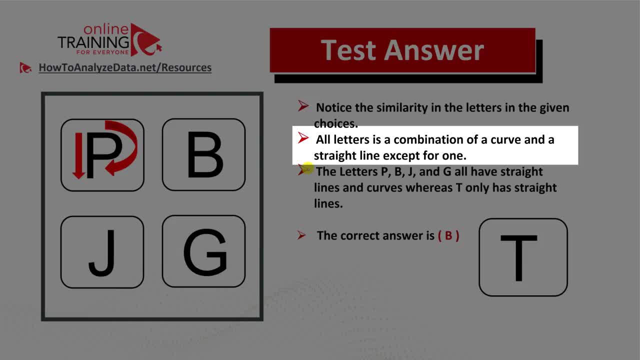 Now let's go ahead and jump to the solution. When you look at the patterns, you can notice the similarities in the letters for the given choices. All letters are combinations of the curve as well as straight line, with the exception of one, The letters P, B, J. 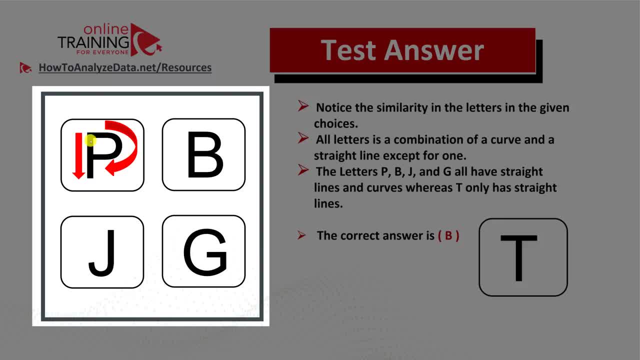 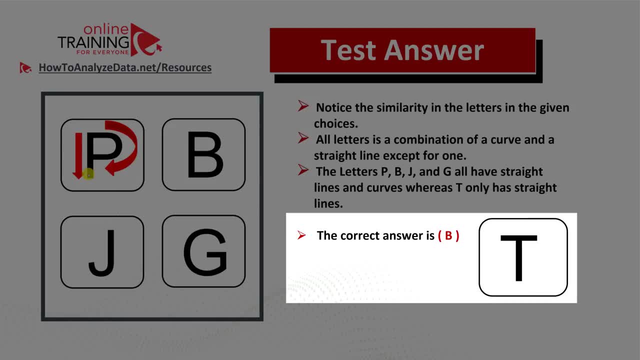 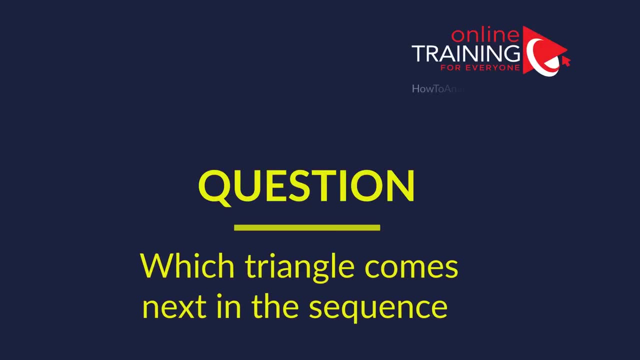 and G presented here. they all have combination of curve as well as straight line. The only letter that does not match this pattern is letter T, So the correct choice here is choice B, letter T. Hopefully you've nailed this question. All right, I have a tricky question for you, which you might frequently see. 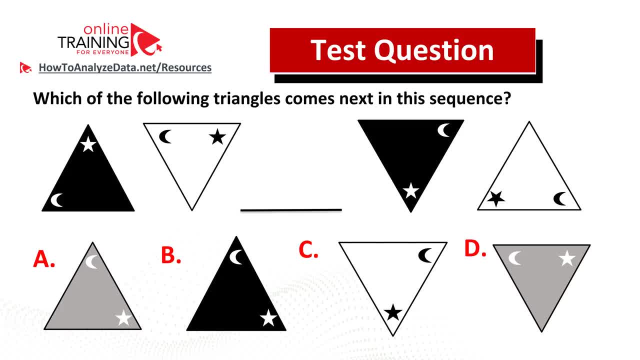 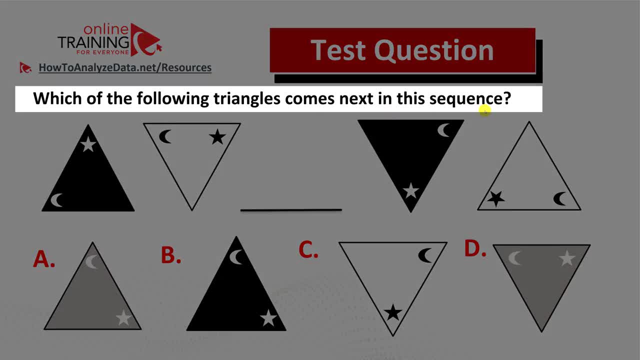 on the test. The cool thing is that you might be able to solve it. or in case you don't, I would love to show you the solution. Which of the following triangles comes next in the sequence? You have sequence of five triangles. 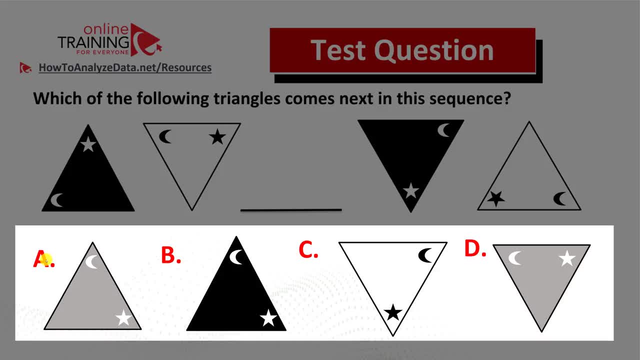 and one triangle in the middle is missing, And you have four different choices to pick the right triangle: Choices A and B, represented by gray and black triangles pointing toward the top, And choices C and D, represented by white and gray triangles pointing to the bottom. 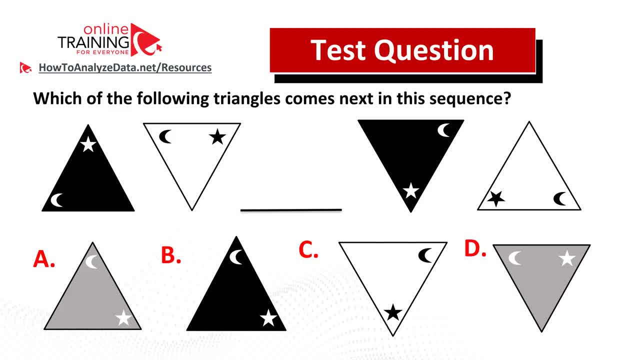 Do you think you know the answer? Now might be the right time to pause this video to see if you can come up with the answer on your own. Do you think you came up with the answer? Let's continue to see how we can solve this challenge. 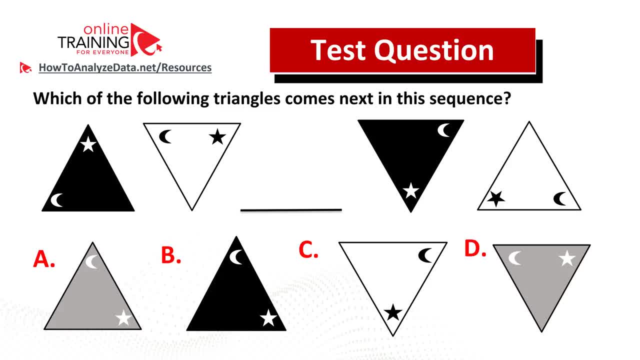 together. Before revealing the solution to you, I would like to point at two patterns that we see in this problem. The first is the pattern of colors. You have black triangle, white triangle and then missing triangle, Then black triangle and white triangle and then missing triangle. 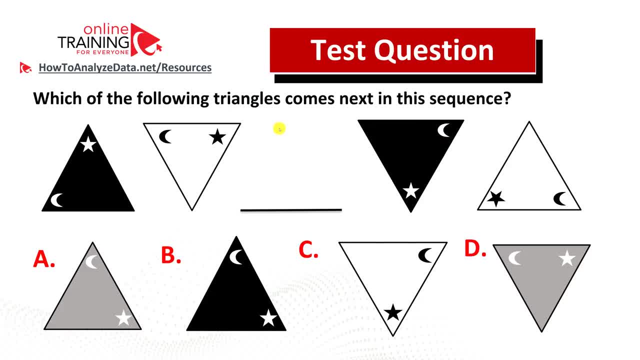 Then black triangle and white triangle. So something might be different from black and white. potentially here You also have a pattern of moon and star And moon and star. they move inside the triangle. So you see moon and star in the leftmost triangle, Then you see moon and star on the top. 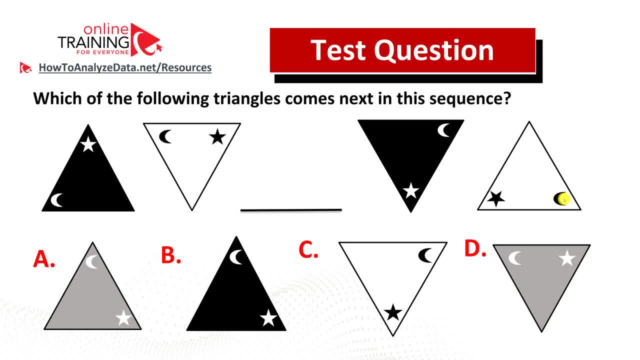 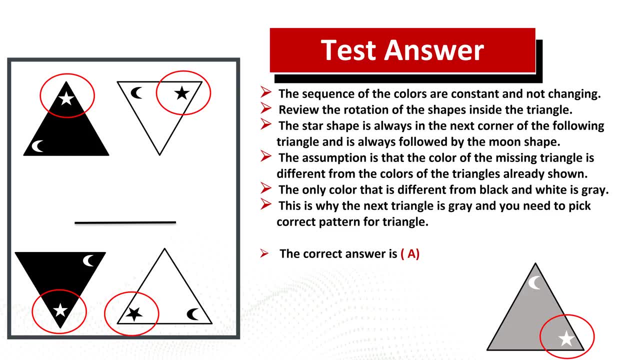 Then you see moon on the top and star at the bottom, And then you see both of them, moon and the star at the bottom of the triangle. So now let's jump to the solution. We have already looked at the pattern of the colors and the sequence of colors is constant, and 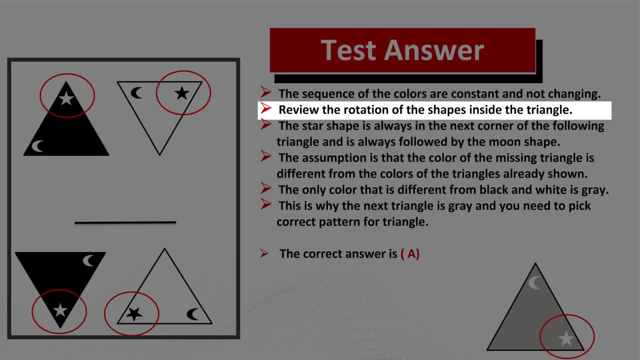 is not changing, And we also reviewed the rotation of the shapes inside the triangle. The star shape is always in the next corner of the following triangle and is always followed by the moon shape. The assumption here is that the color of the missing triangle is different from the colors 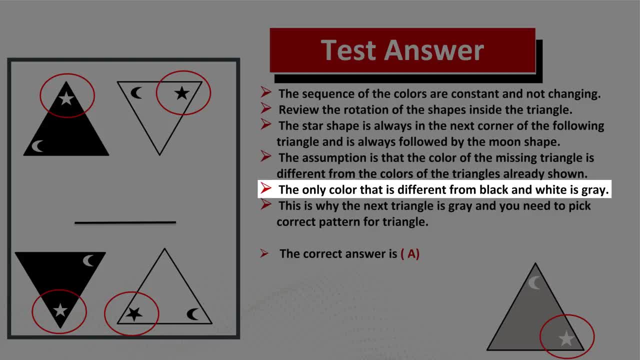 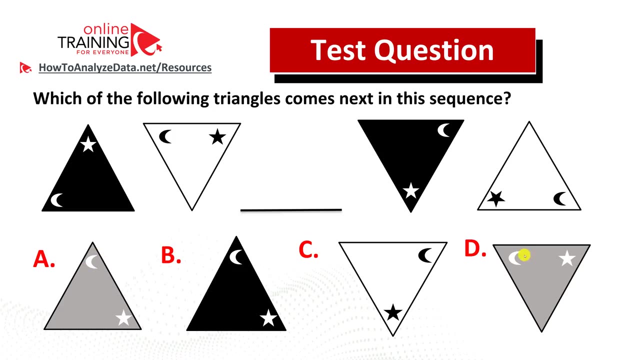 of triangles already shown, And the only color that is different from black and white is gray. The next triangle is gray and you would need to pick correct pattern for the triangle, So the correct choice here is choice A. There are two gray triangles here, Choice A and choice D, But there is also a. 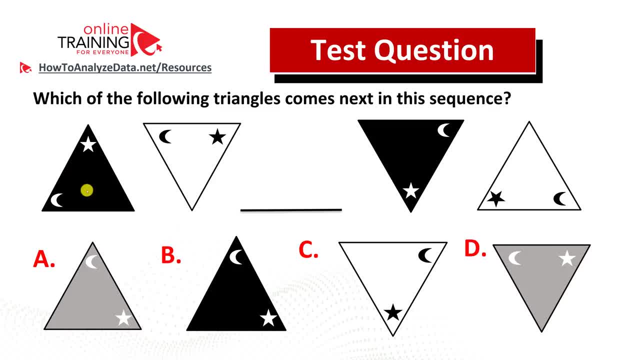 third pattern Pattern that I did not mention because it will make things very obvious, And this is the pattern of pointing. You see that the first triangle is pointing upward, The second triangle points down, So the next triangle in the pattern will be pointing up as well, And the only gray triangle that points up is choice A. 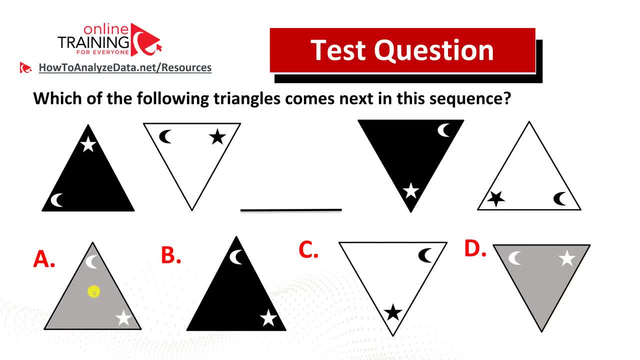 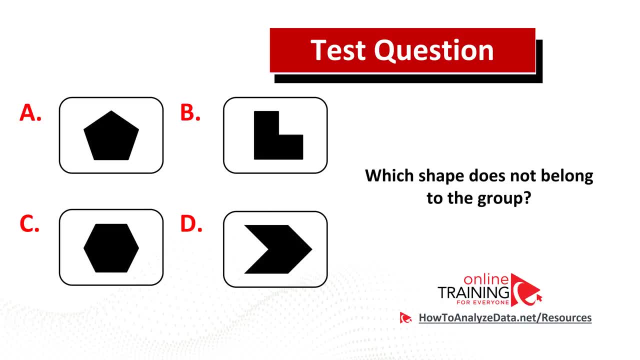 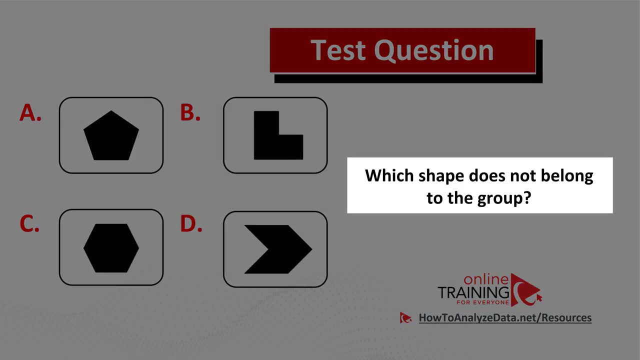 Hopefully you've nailed this question and now know how to see the patterns and solve these types of challenges on the test. And now here is the question for you to try. You can pause this video and try to solve it. Which shape does not belong to the group? And you have four choices. 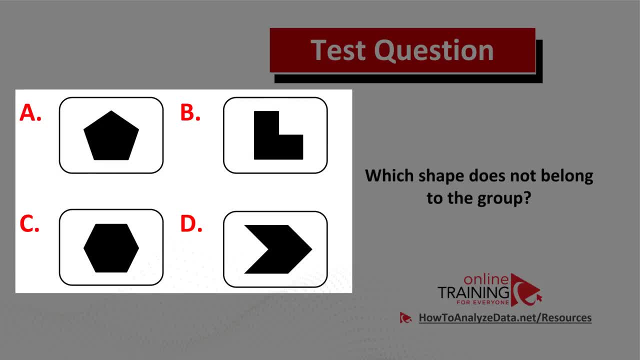 of shapes. Please look carefully at all the shapes and try to determine the one that does not match particular pattern. You can pause the video and try to solve it And if you came up with the answer, feel free to post the answer in the comments So I'll give you my feedback. Thanks for participating. 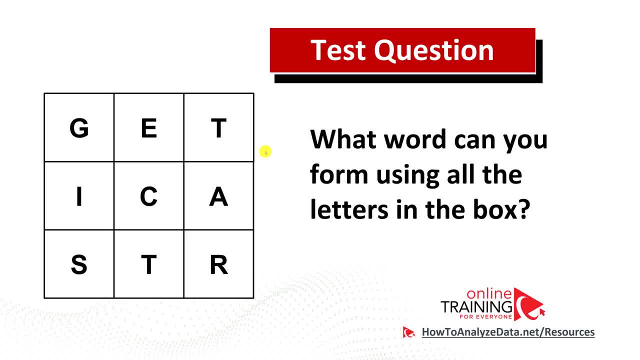 Let's look at the very interesting and at the same time, tricky question you might frequently see on the test. This particular question tests your imagination as well as the knowledge of the English words. What word can you form using all the letters in the box And you have nine unique letters? 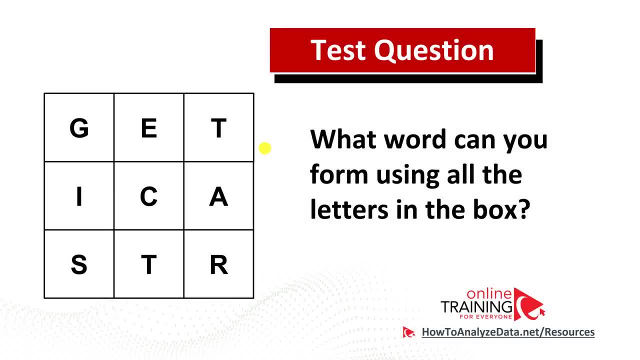 presented in nine different boxes. Do you think you know the answer? Before we jump to the solution, this might be the right time for you to pause this video to see if you can come up with the solution on your own. Do you think you've figured out the answer? Let's continue to see if we can solve this. 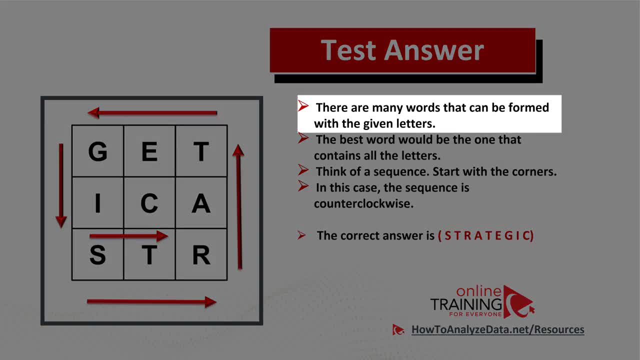 challenge together. Obviously, there are a lot of different words that could be formed with the given letters, But what you need to do as part of the test is to find the word that best matches all the letters presented. You should start looking in the 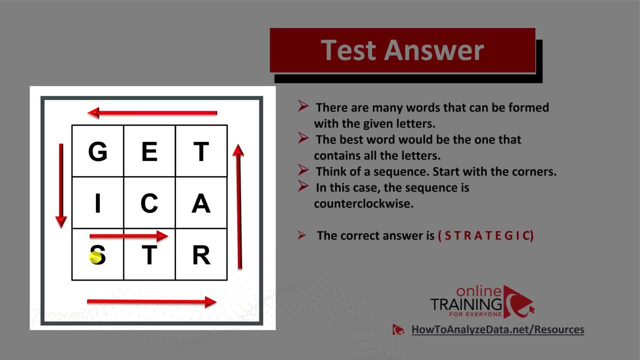 corners and in this case the pattern is counterclockwise. We have the word strategic, which is formed starting in the bottom left corner. If you start in the bottom left corner and then flow from right to left, then flow from bottom to the top, from left to right and then end. 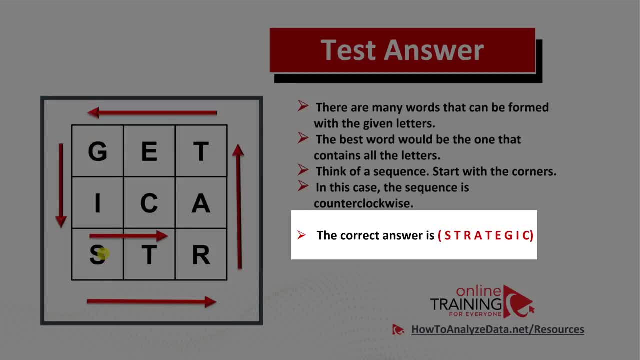 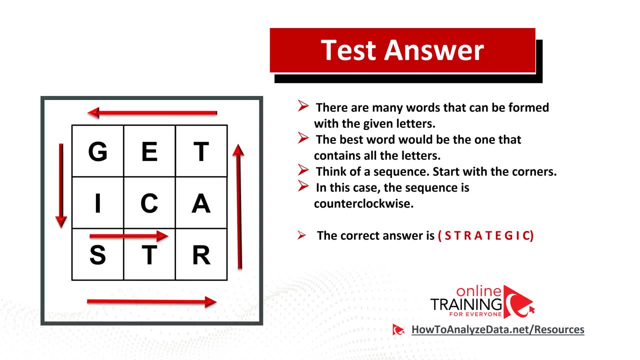 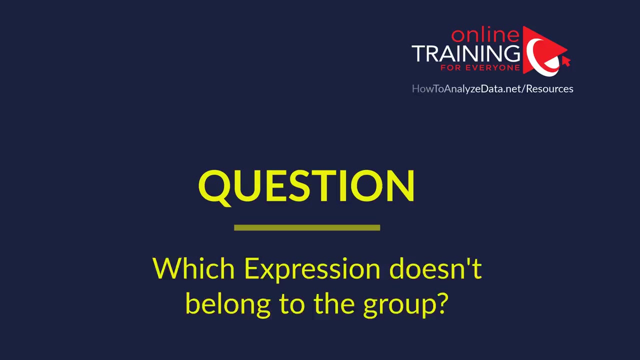 your word in the middle, you will form the word strategic. Hopefully you've nailed this question, but in case you need more questions or practice problems, please make sure to check out the aptitude test book in the description section of this video. Are you ready for this challenging problem? 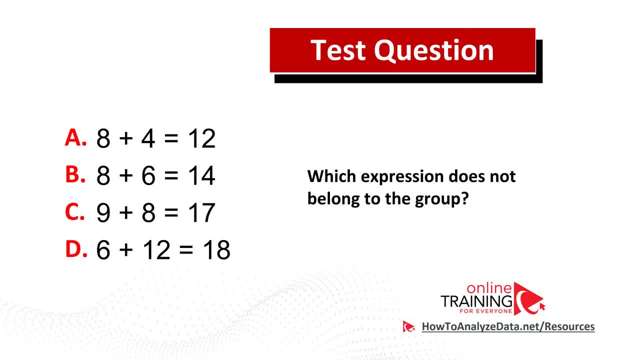 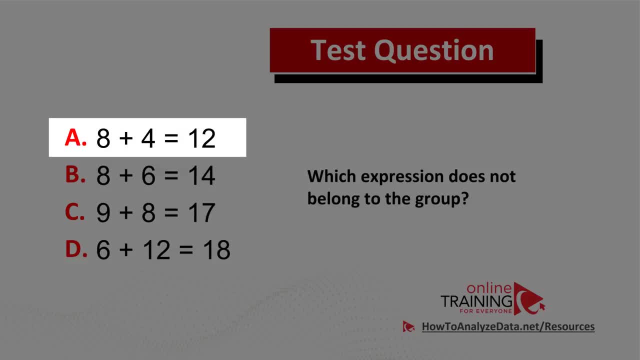 Let's look at the very interesting and tricky question you might frequently see on the test: Which expression does not belong to the group? And you have four different expressions: Choice A: 8 plus 4 equals 12.. Choice B: 8 plus 6 equals 14.. Choice C: 9 plus 8 equals 17.. 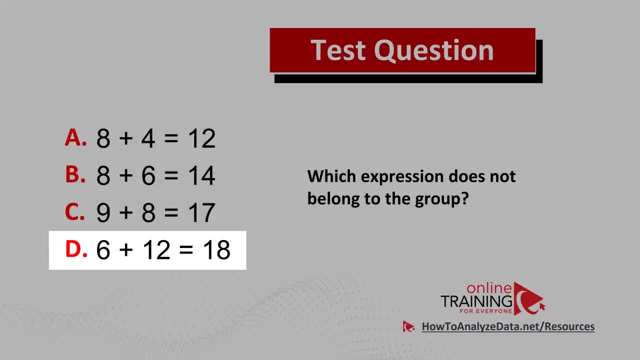 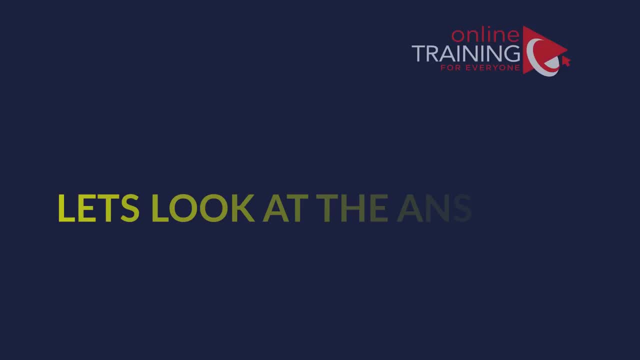 And choice D, 6 plus 12 equals 18.. Do you think you know the answer? Now might be the right time for you to pause the video to see if you can come up with the answer on your own. Do you think you know the answer? Let's continue to see if we can solve this challenge together. 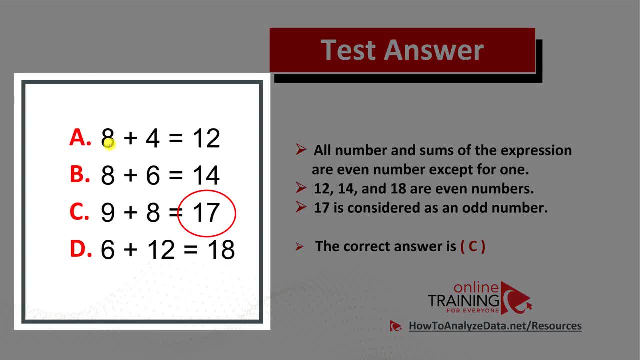 What's interesting about this question is the fact that we're dealing here with odd versus even numbers. You see that expression A has all the even numbers: 8 and 4 equals 12.. Expression B is the same thing: 8 plus 4 equals 12.. And you have four different expressions. Choice C: 9 plus 6 equals. 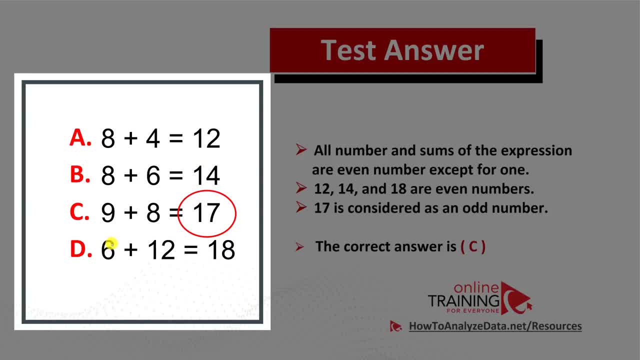 14. All even numbers Same with expression D: 6 plus 12 equals 18.. So the expression C has two odd numbers, 9 and 17.. And if you look at the answers you can also figure it out by just looking at the answer. The answers are 12, 14 and 18 for solutions A, B and D And for the C the answer is: 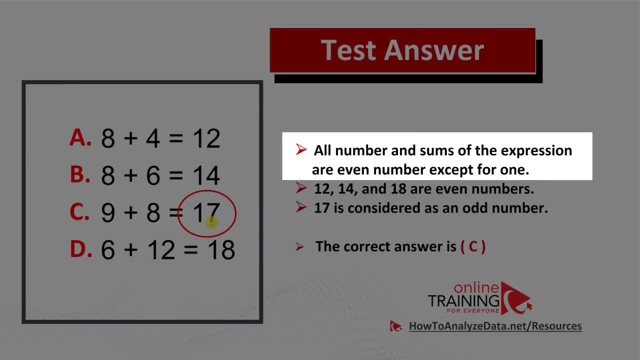 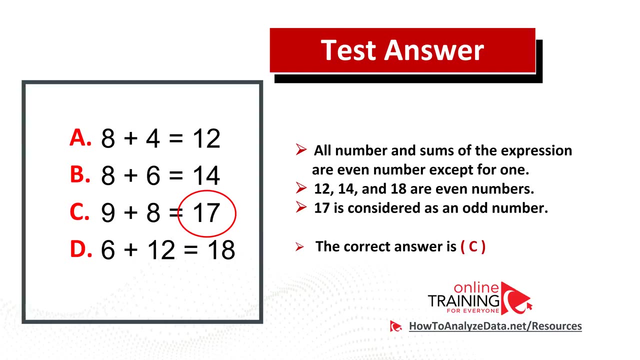 17.. So let's recap: All numbers and sums of the expression are even numbers, with the exception of 1.. 14 and 18 are even numbers, But 17 is the odd number. So the correct answer here is choice C 17.. Hopefully you've nailed this question and got to the correct answer on your own. 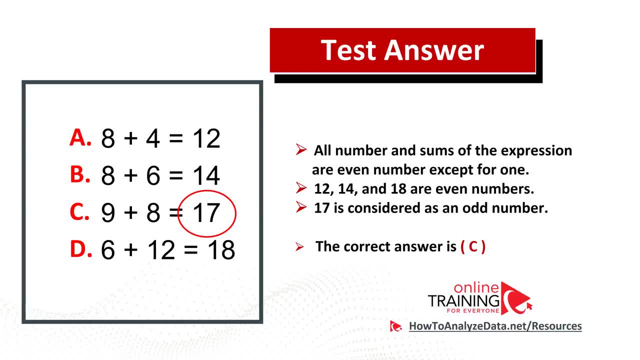 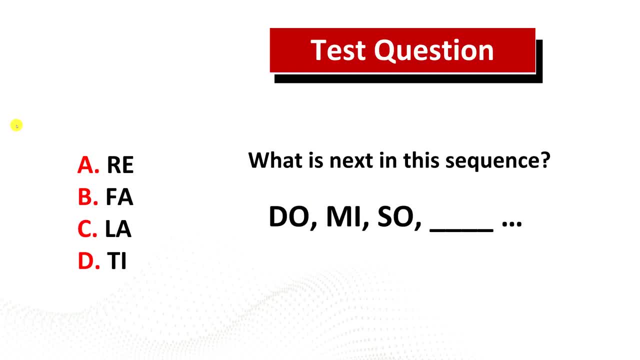 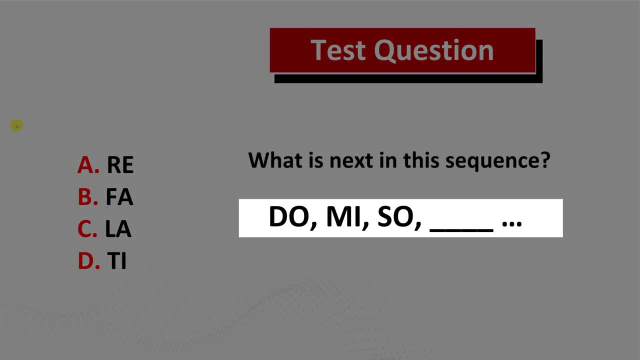 But in case you need more questions or practice problems, please make sure to check out the description of this video for my aptitude test questions pdf ebook. And now here's the question for you to try: What is the next item in the sequence? And you have series of items. 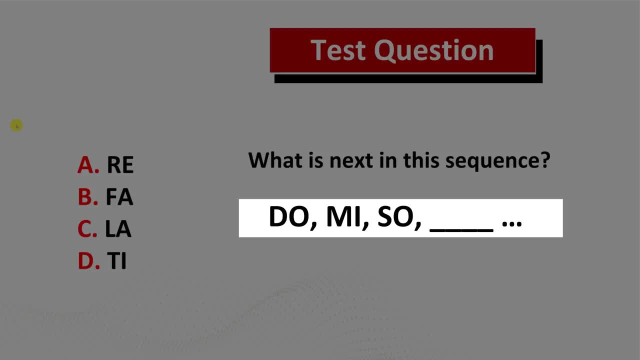 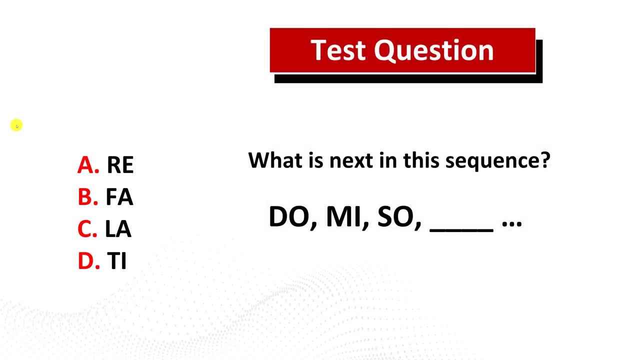 So, me so. and then the next item that you need to determine, And you have four choices: Re fa la ti. Do you think you know the answer? Feel free to pause this video and try to solve it. 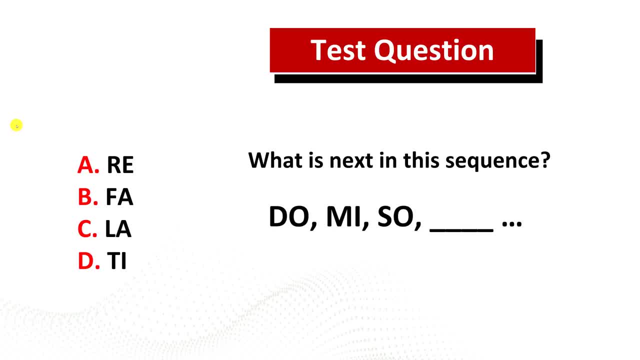 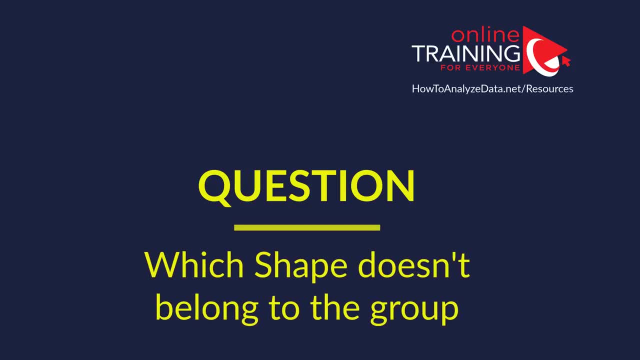 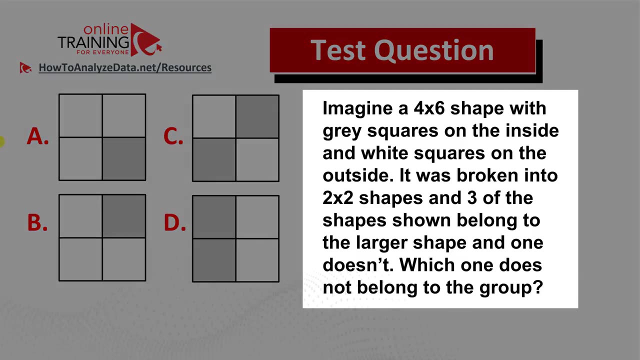 And if you came up with the answer, feel free to post it in the comment section of this video and I'll give you my feedback. Thanks for participating. Here's the tricky IQ and aptitude test question you might frequently see on the test. Imagine a 4x6 shape with gray squares on the inside and white squares on the outside. 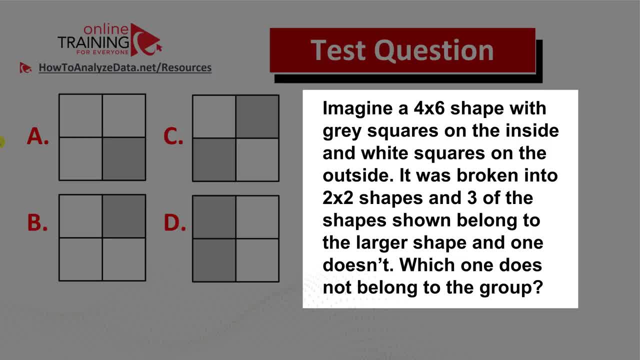 It was broken into two by two shapes, and three of the shapes shown belong to the larger shape and one doesn't. Which one does not belong to the group? Do you think you know the answer? Now might be the right time to pause this video to see if you can come up with the answer on your own. 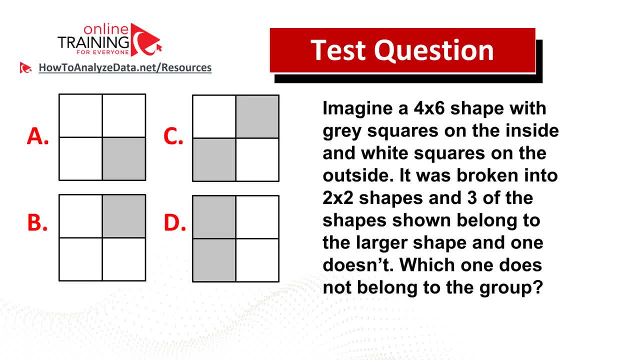 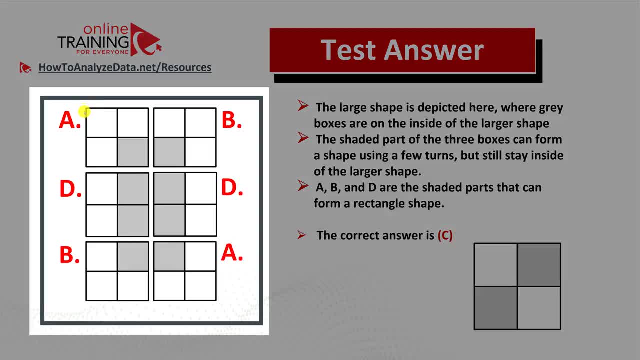 Do you think you came up with the answer? Let's continue to see, see if we can solve this challenge together. As you might be well aware, a visual is worth 1000 words or more. In this case, this is the shape- 4x6 shape- with the gray boxes on the inside and. 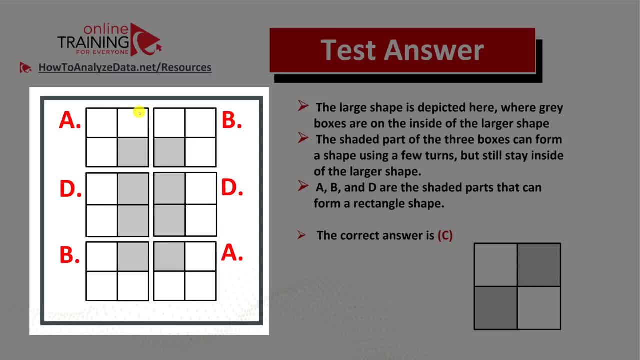 the white boxes on the outside And it was broken down into 2x2 shapes. If we go back to the question, you see that the choice A is represented right here. If you flip the box in the bottom right corner of the screen, choices B are in the opposite corners and choices D are in the middle. 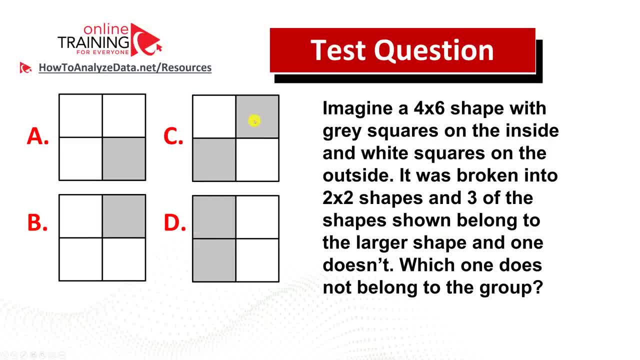 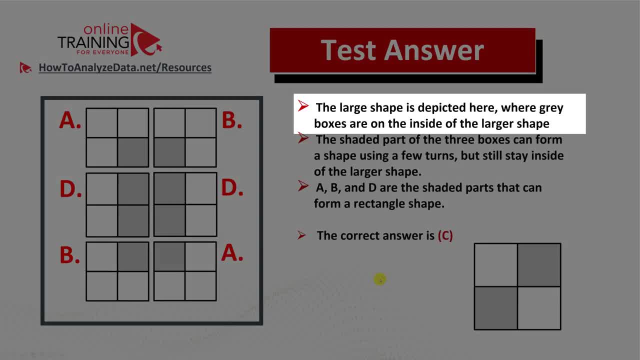 But what you see is that choice C is not represented here anywhere. So the correct answer here is choice C. Let's recap: The large shape is depicted right here, where gray boxes are on the inside and the white boxes are on the outside of the larger shape, The shaded part of 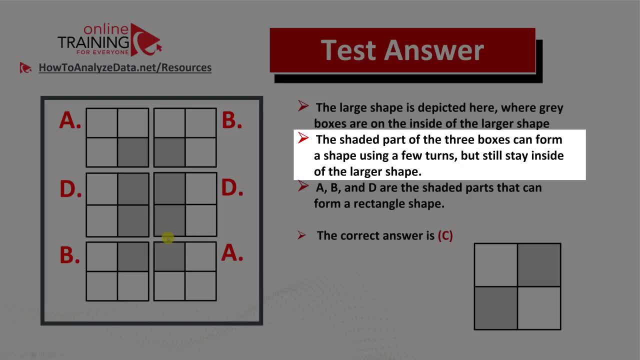 three boxes can form a shape using few turns, but still stay inside the larger shape, The. This is why choices A, B and D are valid choices And choice C is the correct choice And this is the one you should be selecting. 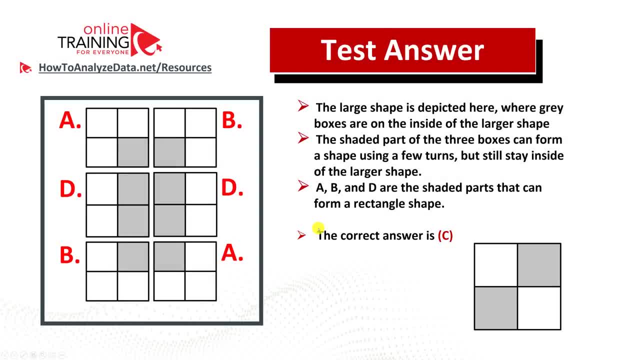 Hopefully you've nailed this question and answered it correctly, But in case you need more questions or practice problems, please make sure to check out my aptitude test question books in the description of this video. And now here's the question for you to try. 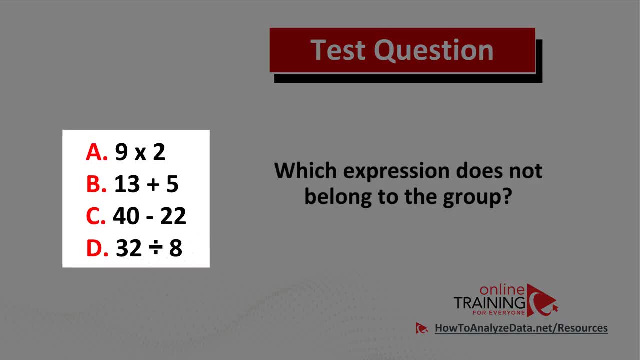 Which expression does not belong to the group. And you have four different choices: 9 by 2,, 13 plus 5,, 40 minus 22, or 32 divided by 8.. Do you think you know the answer? Feel free to pause this video and try to solve it. 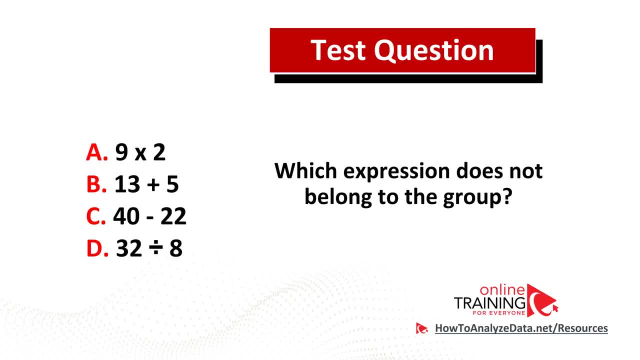 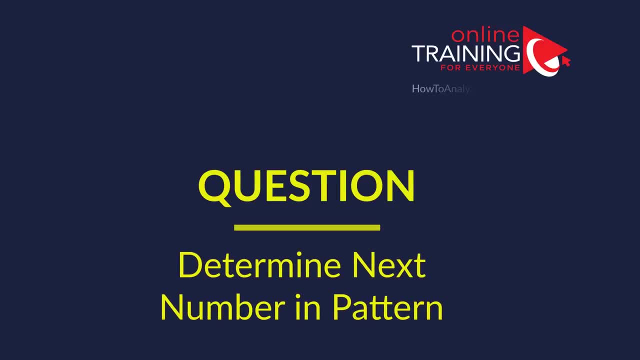 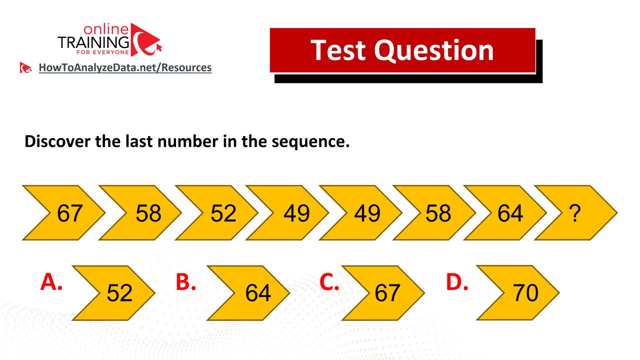 And if you came up with the answer, feel free to post it in the comment section of this video and I'll give you my feedback. Thanks for participating. Let's look at the tricky question you might frequently see on the test. This is the pattern question. 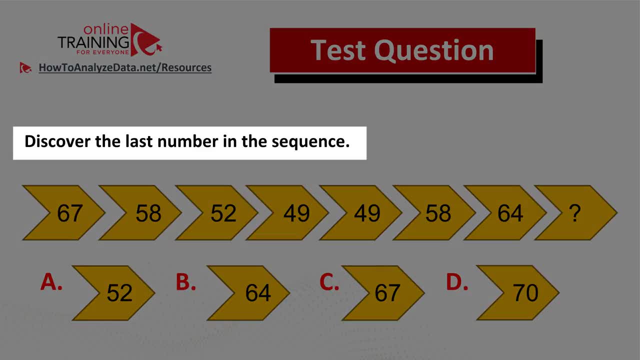 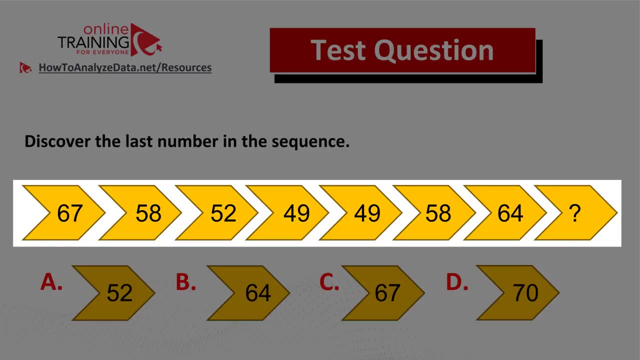 And you need to discover the last number in the sequence. Let's look at the sequence of numbers 67,, 58,, 52,, 49,, 49, again 58,, 64, and then the missing number, And you have four different choices. 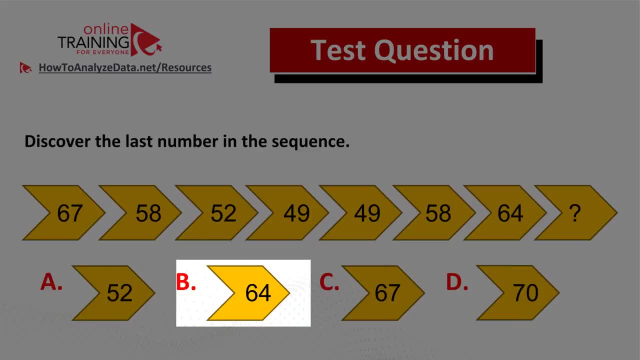 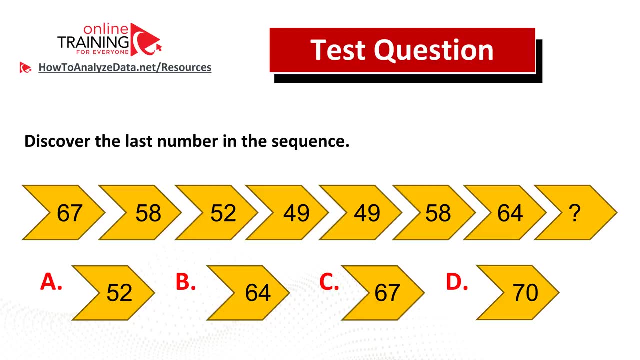 Choice A: 52.. Choice B: 64.. Choice C: 67.. Choice D: 70.. Do you think you know the answer? Now might be the good time to start. Feel free to pause the video to see if you can come up with the answer on your own. 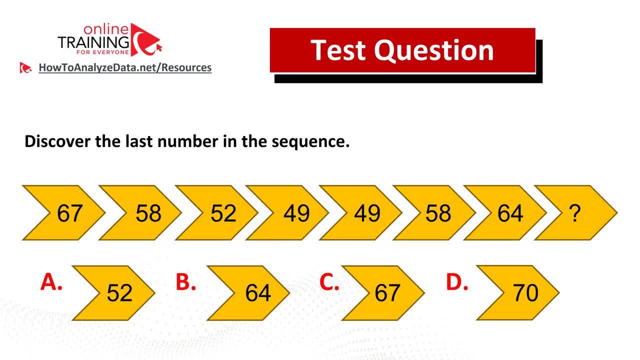 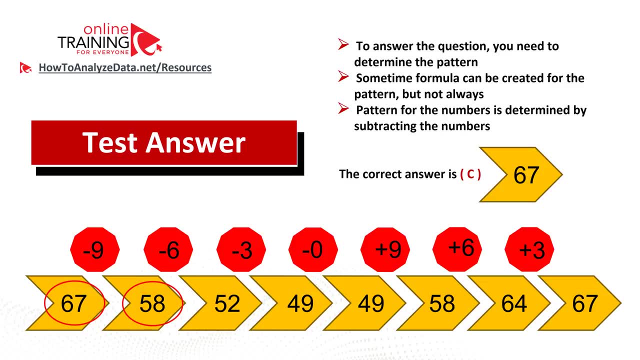 Did you come up with the answer. Let's continue to see if we can solve this challenge together. To answer the pattern question, you need to determine the formula, And a lot of times you can't do that, but not in this particular case. 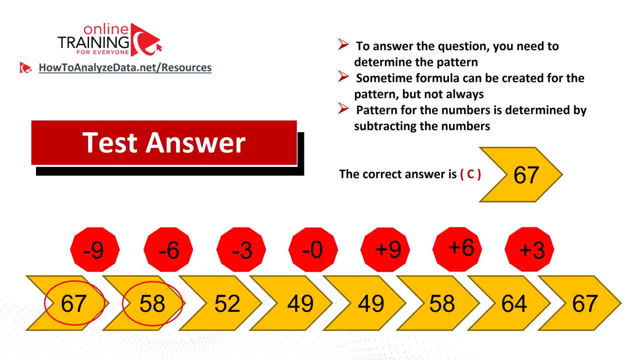 I couldn't come up with the formula for this particular question, but maybe you will be able to, So please make sure to post your answer in the description of this video. But let me share with you my logic and how I came up with the sequence of numbers. 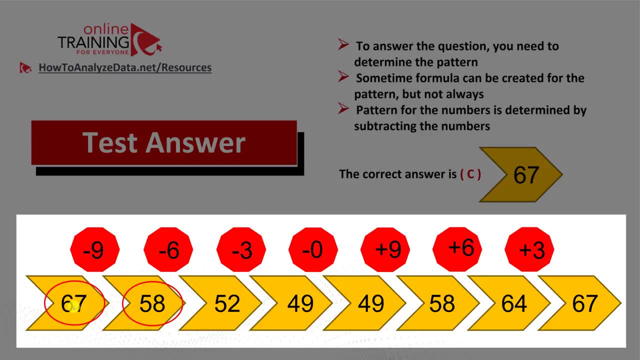 If you look at the series of numbers, for example between 67 and 58,, you see that the difference is minus nine. If we put minus nine on top in between 67 and 58, and then continue and put the differences in between the steps in the numbers, 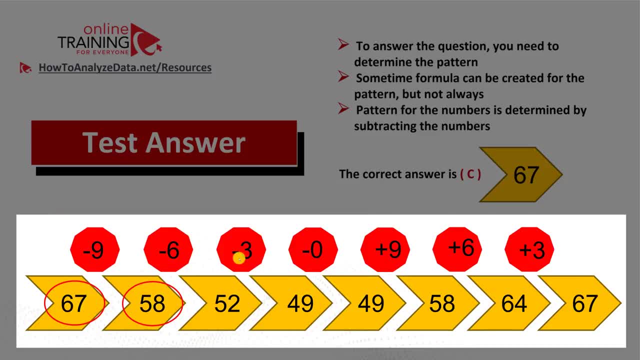 you will see that the differences will account for minus nine minus six, minus three, zero plus nine plus six, and the next number would be plus three, and if we follow the pattern, that would be the next number. And that's how we came up with the answer of 67.. 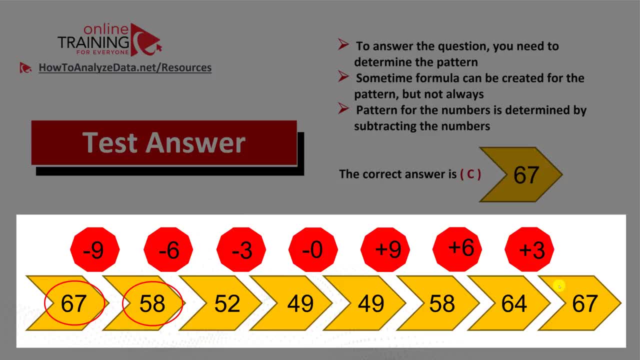 So the tricky part of the pattern questions is that a lot of times there is a formula. but don't spend all your time on the test doing the pattern questions and trying to find the formula. Sometimes all you need to do is just to put the differences on top of the numbers mentally. 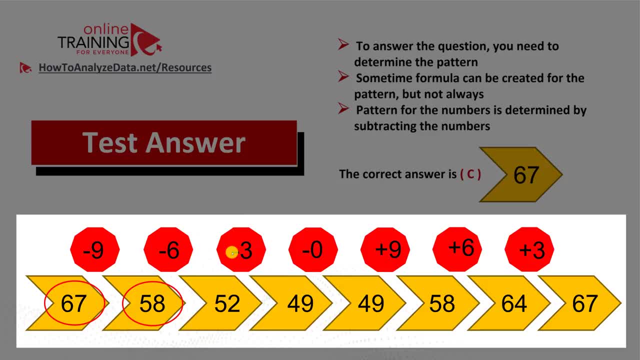 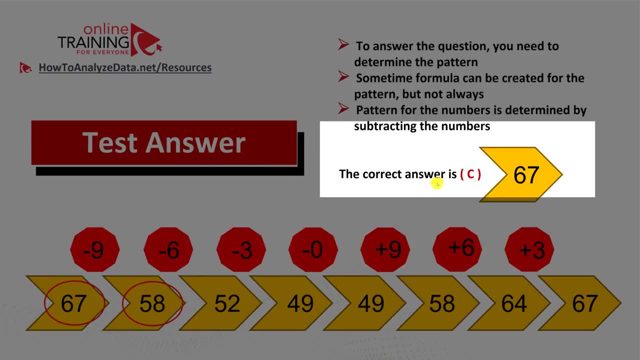 maybe on the piece of paper, and then this will give you the differences in the numbers and you will be able to come up with the final answer. So the final answer here is C 67.. Let's recap: To answer pattern questions, most of the time you need to determine the formula. 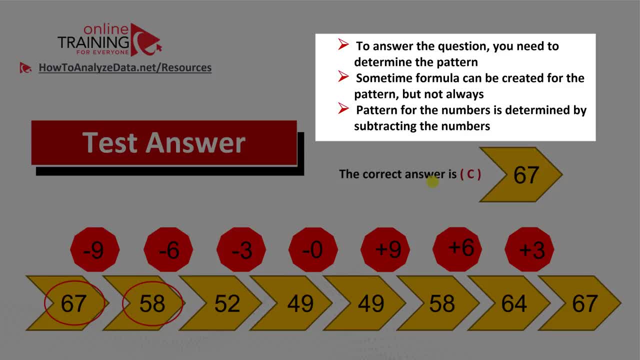 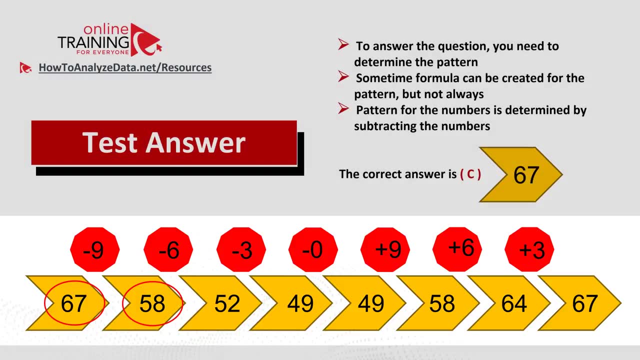 In this particular case there is no formula, So all you need to do is just put the differences between the numbers and determine the last number in the sequence. Hopefully you know now how to answer these types of questions on the test And if you know the formula for this or maybe could come up with the formula- 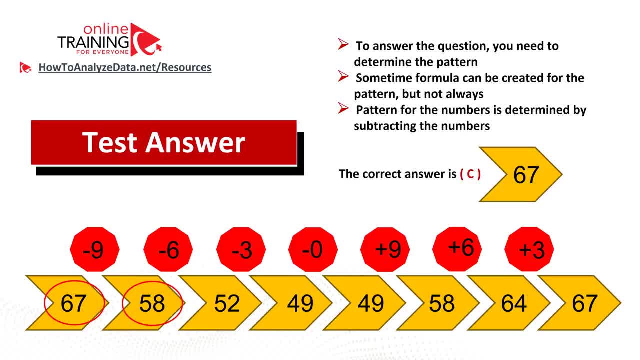 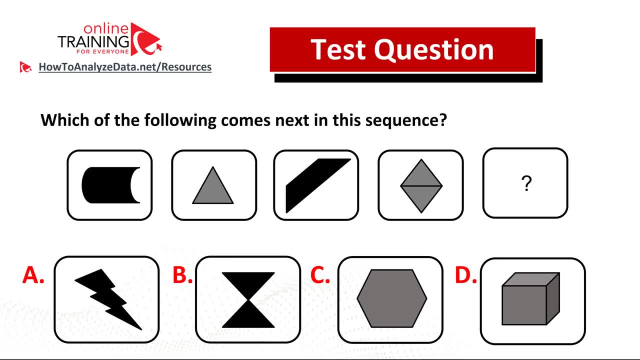 feel free to share in the comment section of this video. And now here's the question for you to try. Please make sure to post your answer in the comment section of this video. You are presented with the sequence of objects and you need to determine which one comes next in the sequence. 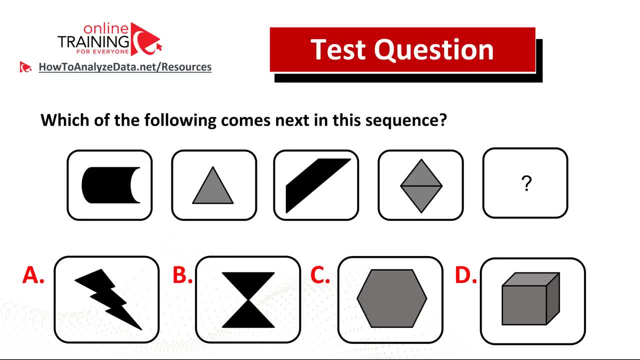 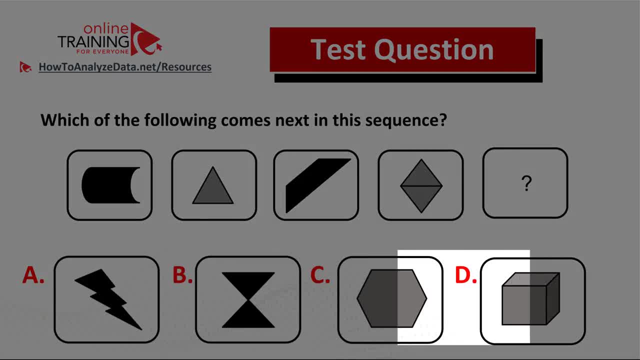 Do you think you know the answer? Now might be a good time to pause this video and to see if you can come up with the correct answer. Is it lightning sand, clock, hexagon or cube? If you came up with the answer, feel free to post it. 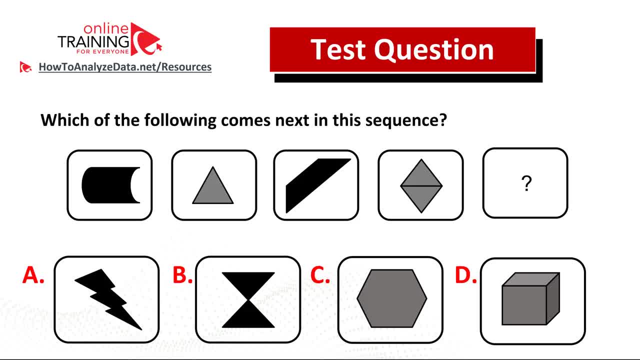 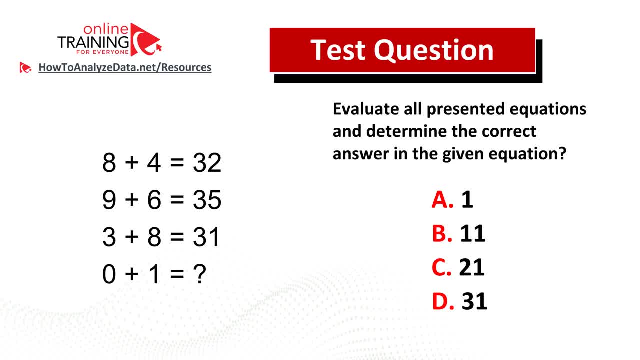 Let me know in the comment section of this video and I'll give you my feedback. Thanks for participating. This question is quite tricky, but I'll show you the solution. Let's solve this challenge together. Here is a very interesting and tricky question you might frequently see on the test. 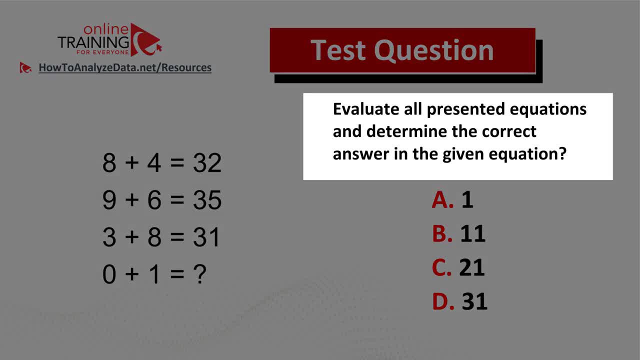 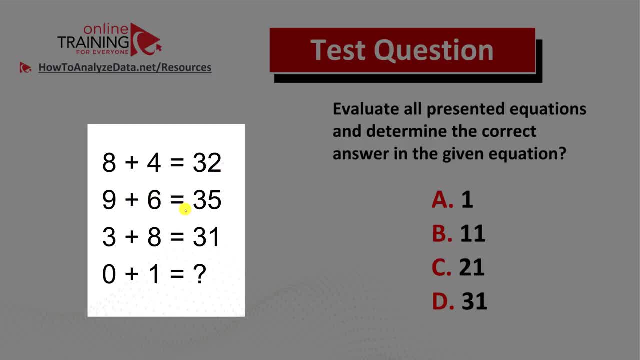 So you have four equations presented: 8 plus 4 equals 1.. 9 plus 6 equals 35.. 3 plus 8 equals 31.. And 0 plus 1 equals something. And you have four possible choices. Choice A: 1.. 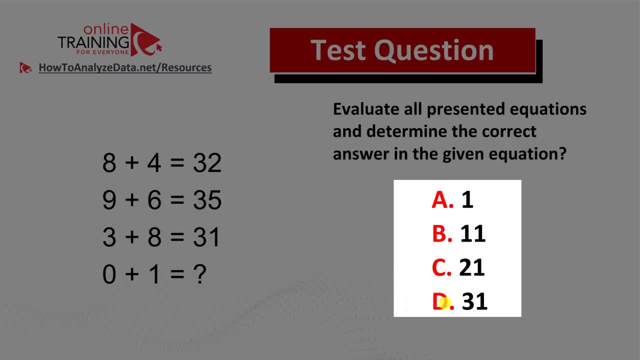 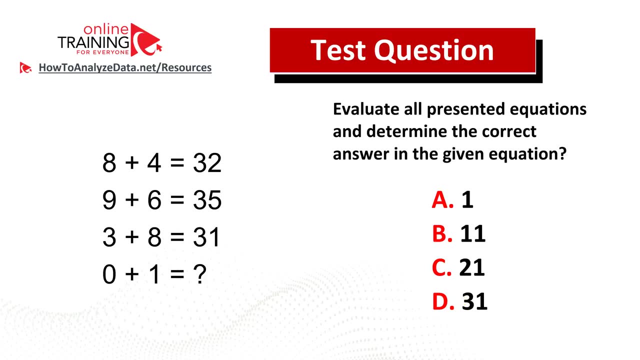 Choice B: 11. Choice C: 21. Choice D: 31. Do you think you know the answer? Now might be a good time to pause this video to see if you can come up with the answer on your own. Did you come up with the answer? 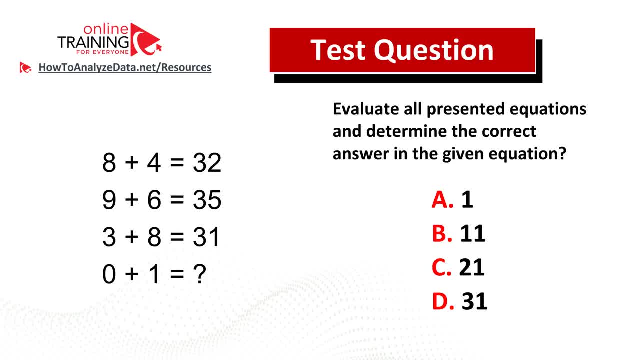 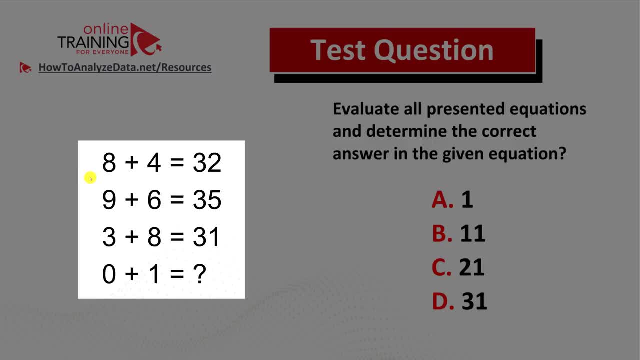 Let's continue to see how we can solve this challenge and get to the solution together. Before we jump to the solution, let me give you some tips. It is still a decimal system that we're dealing with here, And if we continue with this assumption, we can see that the sum of numbers in all cases is a little bit higher than the actual numbers in the decimal system. 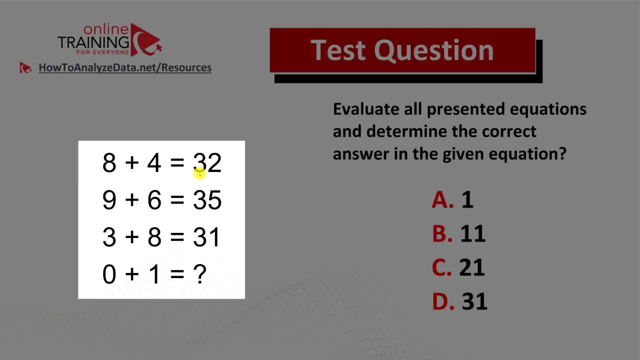 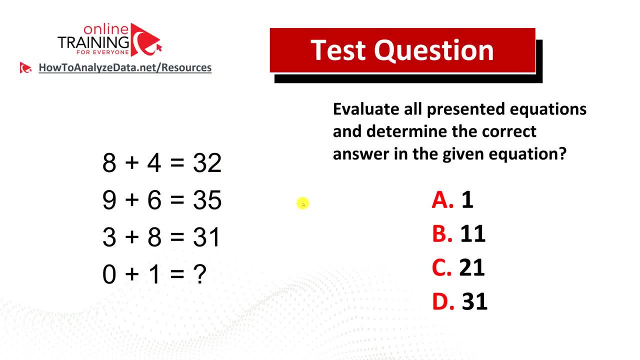 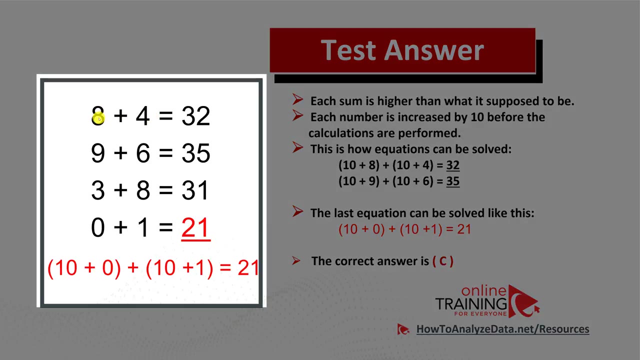 8 plus 4 in reality is 12, not 32.. But the difference between 32 and 12 is still there. 32 and 12 is 20.. Hopefully this gives you some tip. Now, continuing with this logic, basically what's happening is that each number is incremented by 10 before the calculations are performed. 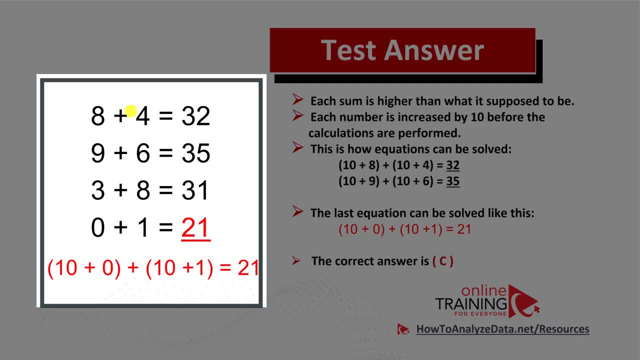 For example, 8 plus 10 is 18 and 4 plus 10 is 14.. 18 plus 14 equals 32.. Same calculations are done with the second, third and fourth equations. For example, 19 plus 16 equals 35.. 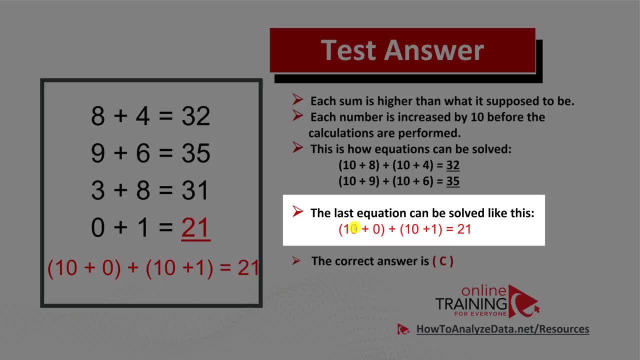 And the last equation can be solved like this: 10 plus 0,, 10 plus 1 equals 10 plus 11 equals 21.. So the correct choice here is choice C 21.. Hopefully by now you know how to answer these types of questions in the test. 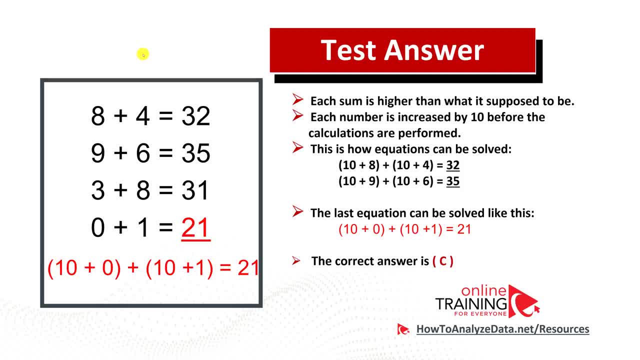 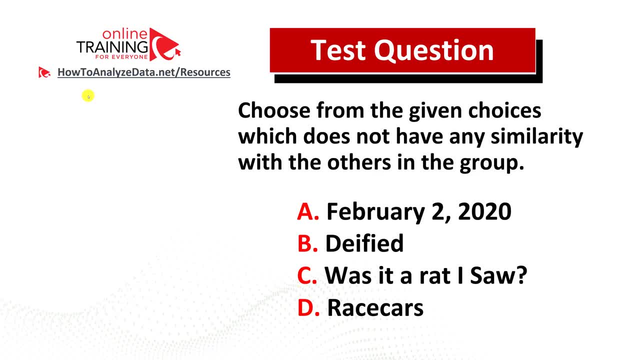 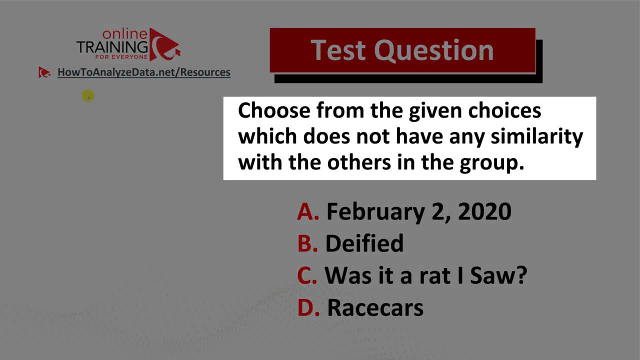 But in case you need more questions or practice problems, please make sure to check out my aptitude test ebook in the description section of this video. And now here's the question for you today. Here's the question for you to try. Please choose from the given choices and identify which item does not have any similarity with the others in the group in your four different choices. 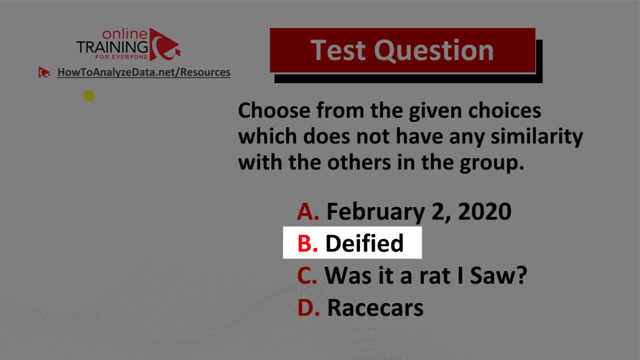 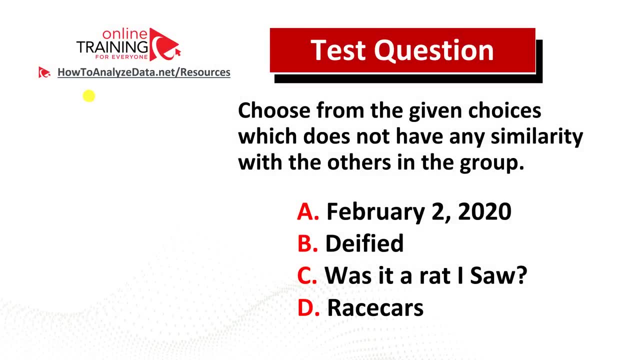 February 2, 2020.. Day 5.. Was it a rat? I saw Race cars. Do you think you know the answer? Feel free to pause this video and try to solve it And if you came up with the answer, feel free to post it in the comment section of this video so I can give you my feedback. 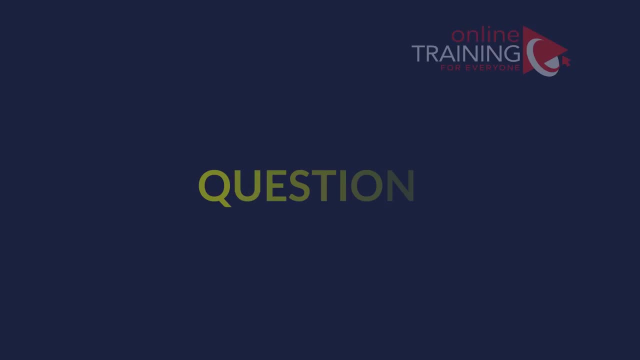 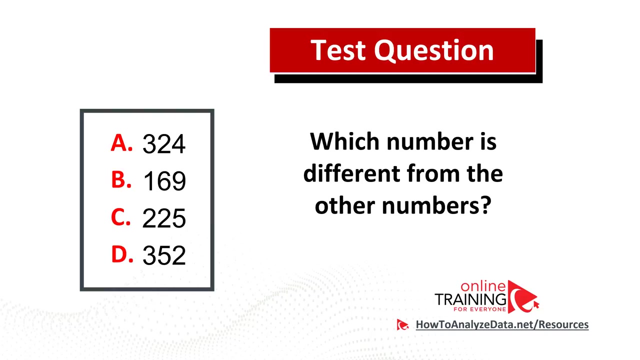 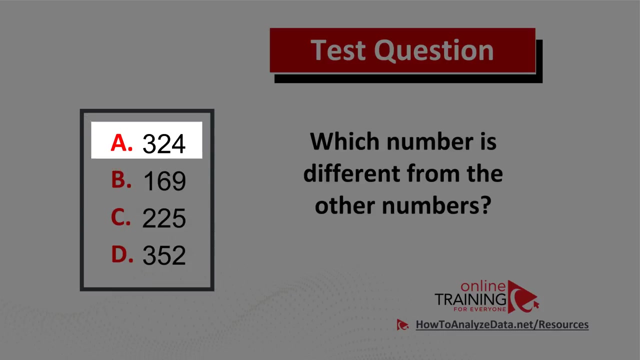 Thanks for participating. See you soon. Let's look at the interesting and tricky question you frequently see on the test: Which number is different from the other numbers in your four different choices? Choice A: 324.. Choice B: 169.. Choice C: 225.. 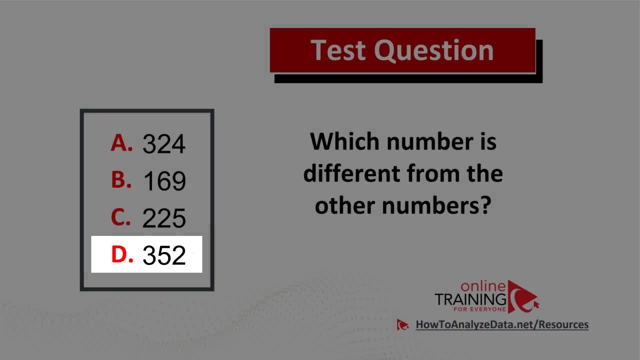 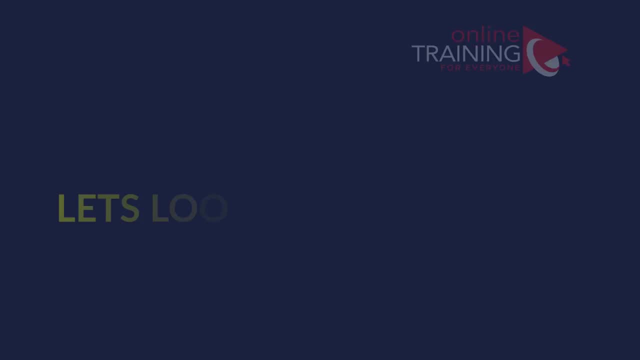 And choice D 352.. Do you think you know the answer? Now might be a good time for you to pause the video to see if you can come up with the answer on your own. Did you come up with the answer? Let's see if we can get to the solution together. 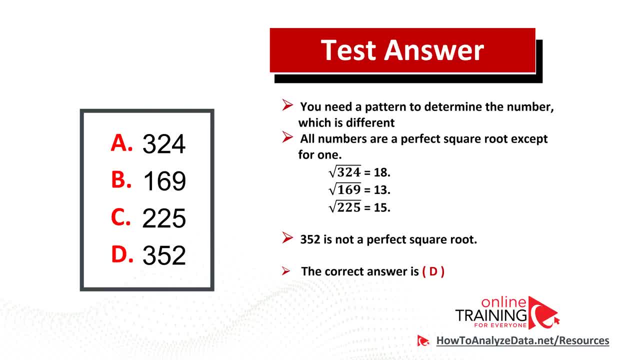 As usual, to get to the answer you need to determine the pattern and understand which three numbers match the pattern and which one number does not belong to the pattern. In this case, the pattern is square root- All numbers here. you can see that three numbers listed here are a perfect square root.